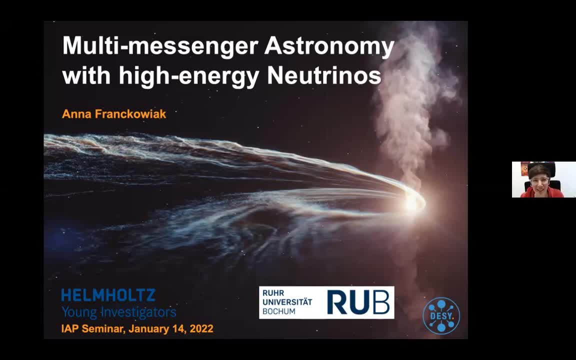 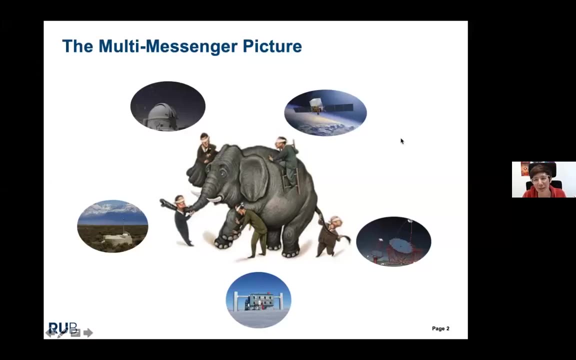 couldn't come in person. I would have much preferred that- But yeah, I do my best to anyway give you an overview of the work I'm doing on multi-messenger astronomy with high-energy neutrinos. So yeah, let me first explain to you the multi-messenger picture and I like to use 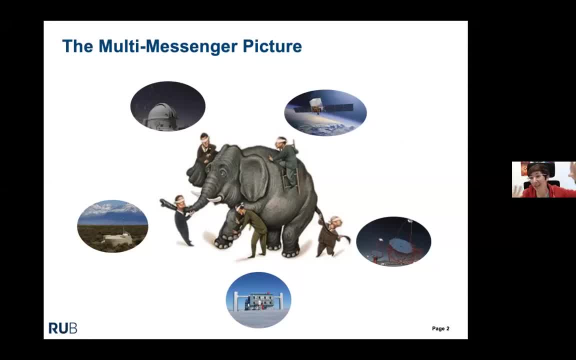 this picture of an elephant and blind man touching the elephant, trying to find the animal they're actually dealing with. And since they only touch a very certain part of the elephant, they will never figure out what animal this actually is if they don't talk to each other. 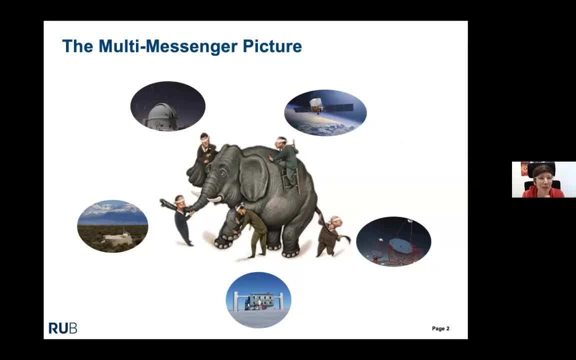 and exchange the data to get a more complete picture, And I think the same is true also for the universe that can be observed in different wavelengths and different messengers. We have to talk to each other and combine all our data to get a more complete picture and understand. 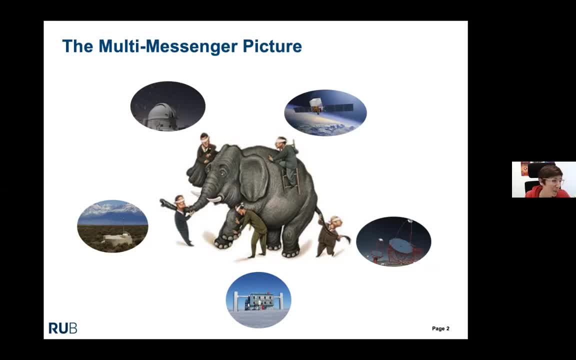 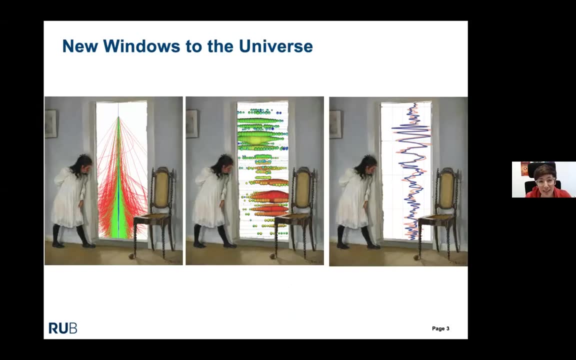 the processes That are happening in the universe. While classically we do astronomy with light, in the recent years we have also added different messengers to this picture, and those are high-energy cosmic rays, neutrinos and gravitational waves, And in my talk I will now focus on the high-energy neutrino part, but of course those are tightly 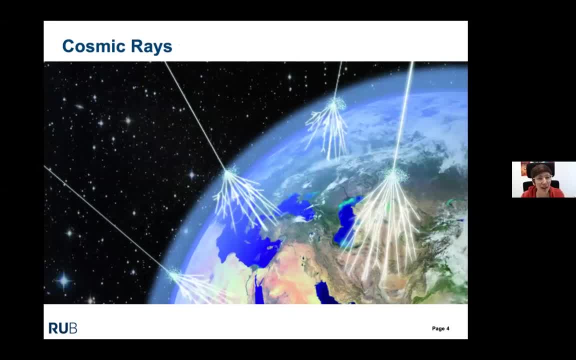 connected to cosmic rays, And cosmic rays are charged particles, mainly protons, that are that bombard us on Earth from all directions all the time And we can measure them and we can measure their energy and we realize that they reach incredibly high energies If we compare this to: 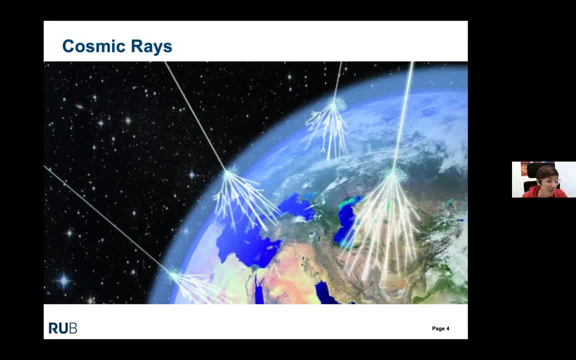 what we can do at LHC. it's 100 million times higher energies that we find in those particles compared to what we can do with our biggest man-made accelerator. So the cosmic rays tell us that they have to be. there has to be incredible. 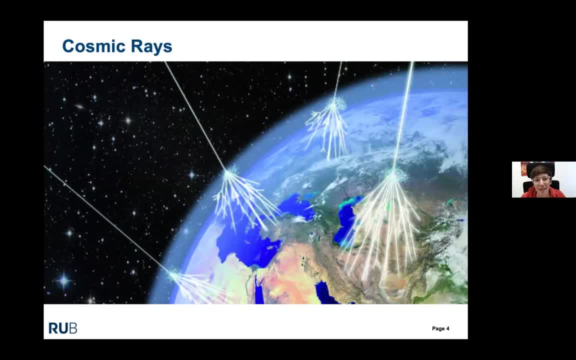 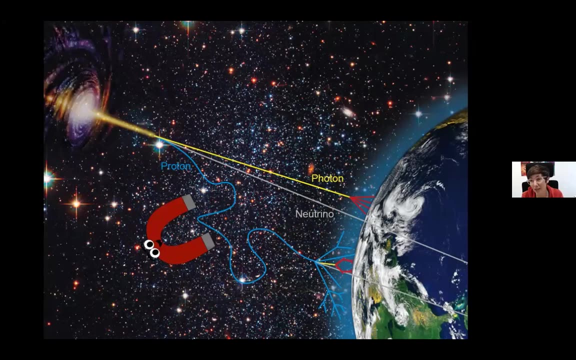 energetic natural accelerators in the universe. So of course we want to find out what are those accelerators, which sources are able to accelerate particles to such high energies? The problem here is if we look at the cosmic rays themselves, because they are charged particles on the way. 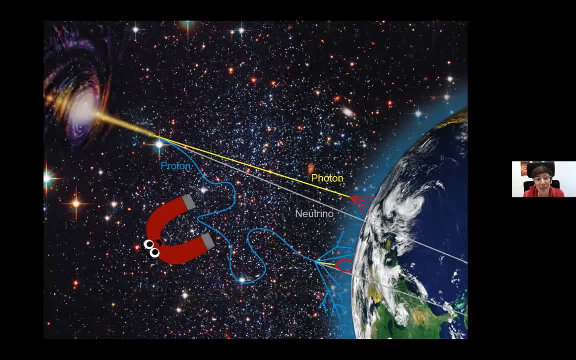 from the source to us. they will be deflected by magnetic fields, So once we measure them on Earth, they don't really point back to their source anymore. And this is where the neutrinos enter the game, because neutrinos- high-energy neutrinos- are only produced. 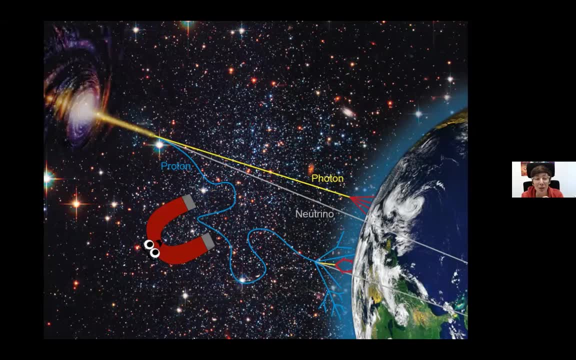 in processes related to high-energy cosmic rays. So, and neutrinos are neutral particles so they can travel straight to us. So if we measure the neutrinos on Earth we can point back to the origin, and this origin also has to be an origin of cosmic rays. Now the neutrinos tell us: 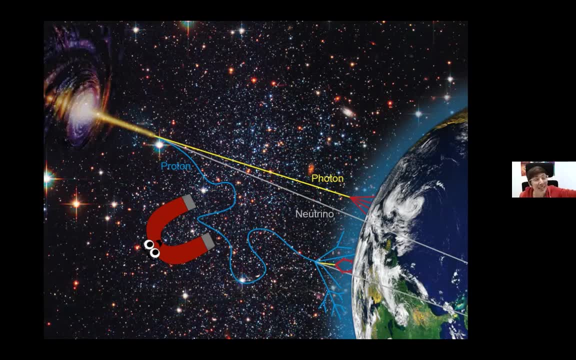 the direction, but now we want to figure out what kind of source is in that direction. So we also need neutrinos in addition to tell us what actually we are looking at there. So some more details on how we actually produce neutrinos. 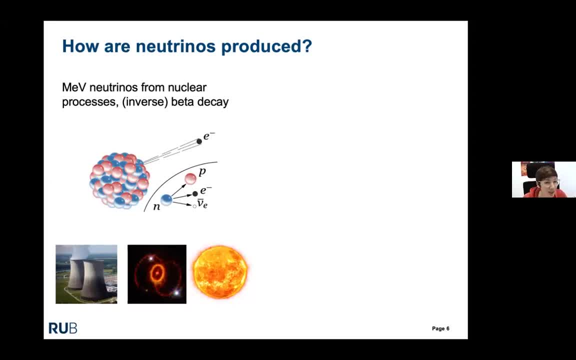 We can have MEV neutrinos that are produced in nuclear processes. We have first measured neutrinos this way in nuclear by next to a nuclear power plant. but we have already then seen them now from the universe. We've seen them from the sun and we've seen them from supernova. 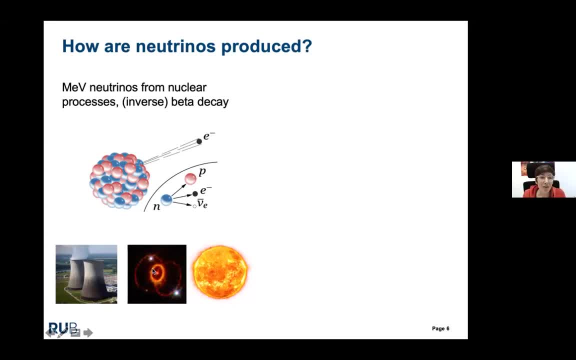 1987A. However, those are not the neutrinos I want to cover today in my talk. So I want to go to much, much higher energies, to TeV and PeV energies, and those neutrinos are produced not in nuclear. 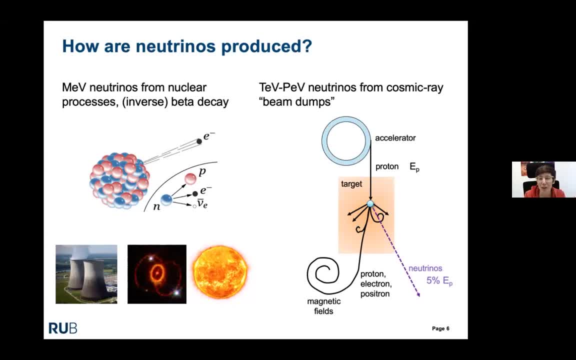 decay processes, but they're basically produced in cosmic ray beam dumps in the universe. So what we need to produce those high-energy cosmic rays are basically two ingredients. We need an accelerator to accelerate protons or heavier nuclei to high energies, and then the 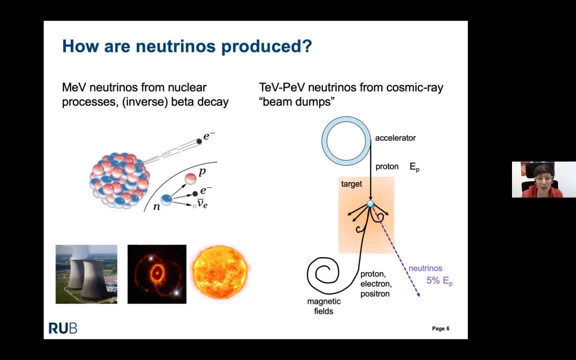 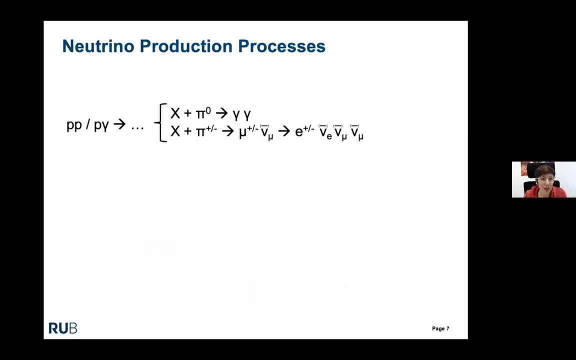 high-energy particles have to interact with some target- That could be matter or a photon field- and in those interactions they will produce high-energy neutrinos And typically then the neutrino takes five percent of the parent proton energy with it. So in some more detail, 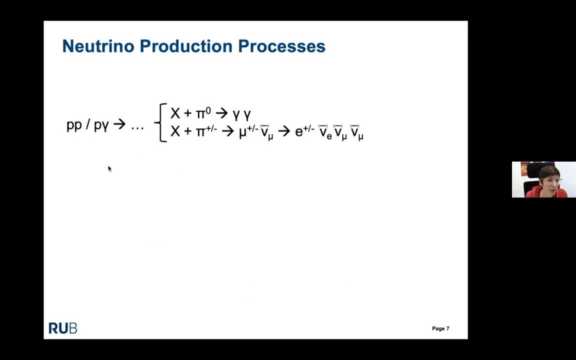 how does the neutrino production look like? I already told you that you need high-energy protons, and then those could interact either with other protons or with photons. Then you produce a bunch of particles, And among those would be pions charged and neutral pions. The neutral pions decay to gamma. 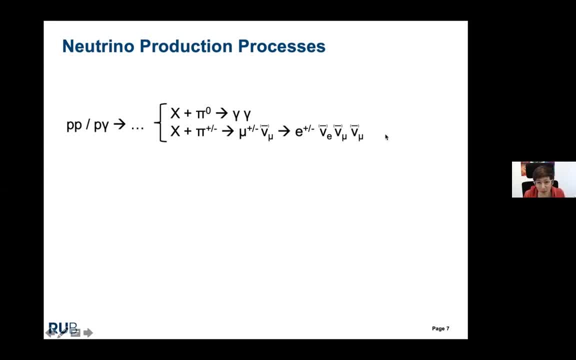 rays, while the charged pions decay to several neutrinos in their decay chain. So now you could ask me: why don't you just look for gamma rays if you want to trace high-energy cosmic rays? And the answer is that gamma rays are not exclusively produced in hydronic processes. 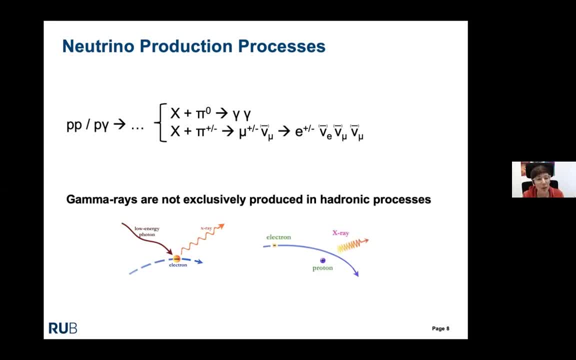 so in processes involving protons. They can also be produced by electrons, for example in inverse Compton and Strahlen processes. So really neutrinos would be the smoking gun signature for hydronic acceleration, because they can only be produced in 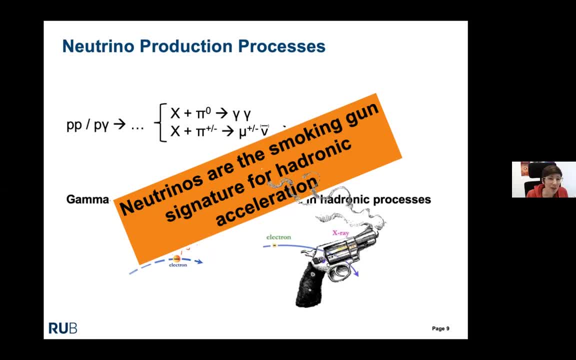 processes involving high-energy protons. That's the main reason why we care about detecting high-energy neutrinos, So they're really unique messengers from the high-energy universe. However, at the same time, they're also very difficult to detect, because they're 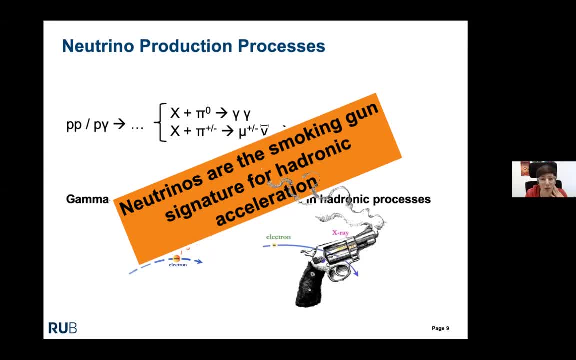 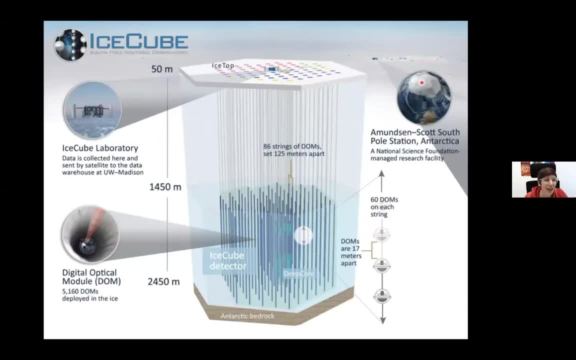 only interact weekly, So either you have to wait really long to catch a few of them or you need a giant detector volume to be able to see a few neutrinos, And the currently largest operating neutrino detector in the world is the IceCube Observatory. 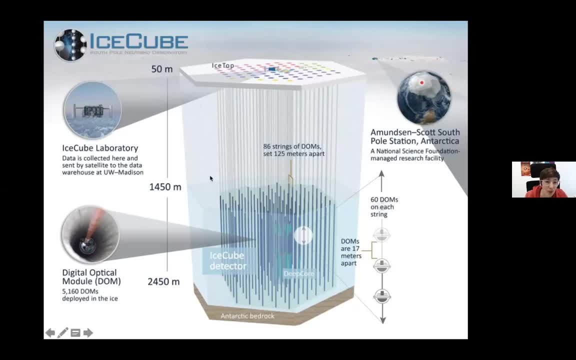 at the South Pole And it's actually a cubic kilometer of the clearest ice in Antarctica, instrumented with more than 5,000 optical modules to detect, actually, the Cherenkov lie that is produced by secondary charged particles produced in neutrino interactions. So basically, we have a particle detector in the ice And what you see? 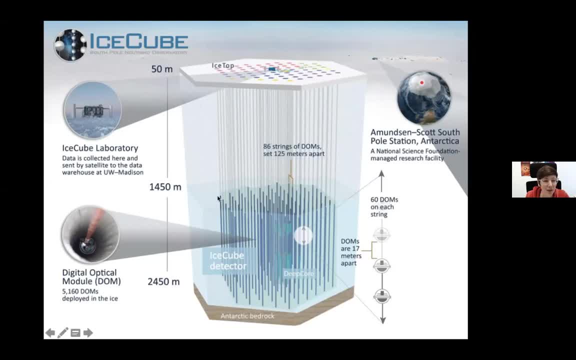 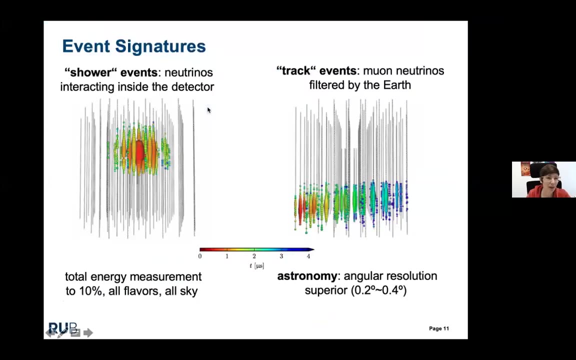 here. so the actual instrumentation starts only one and a half kilometer below the surface, And this is because we have some ice on top of the detector to protect us from background, from cosmic rays. And so how does it look like When we find a neutrino interaction in our detector? here I show two different event. 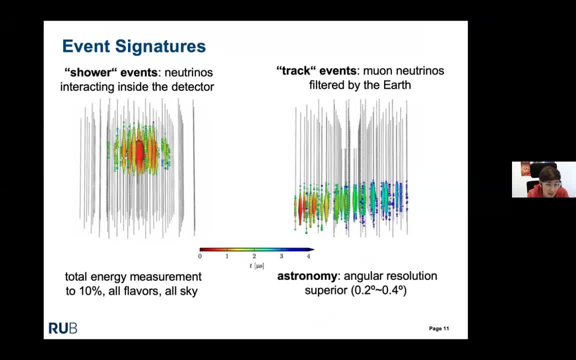 signatures And we distinguish between shower events and track events. The shower events you get from interactions of electron-automne, neutrinos or neutral current interactions. In that case you produce a particle shower in the detector, but the extension of the particle shower is only. 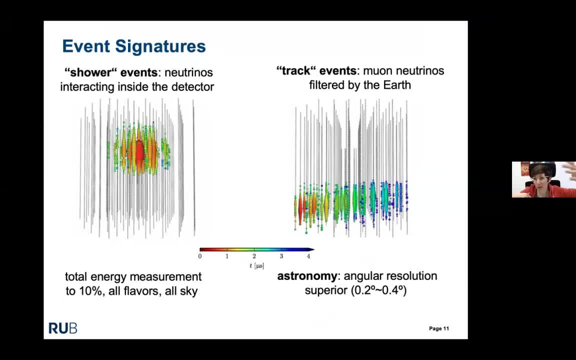 a few meters And if you compare that to the distance between our instrumentation, which is more like a hundred meters, then we cannot really result. The direction of the shower. so we see more a spherical blob of Cherenkov lie. So those events. 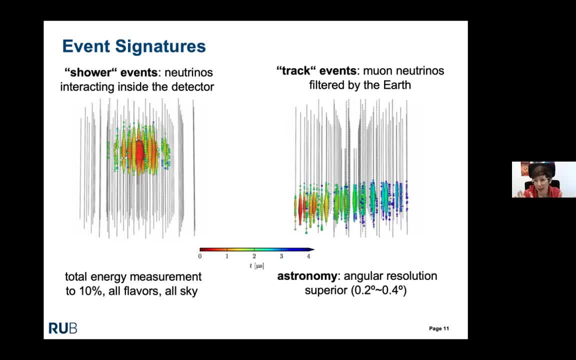 are nice if we want to measure the energy, because most of the lie is contained inside the detector and the lie is a tracer for the energy. However, if we want to get the direction of the event, those shower events are not very suitable. And I should add that each of these colored little 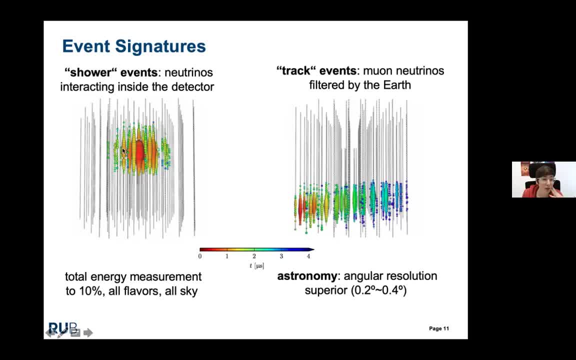 blobs. here is one optical module that's hit by Cherenkov photons And the different colors indicate different arrival time of the light and the different size show how much light, so how much charge which was deposited at the photomultiplier. So the other event type are the: 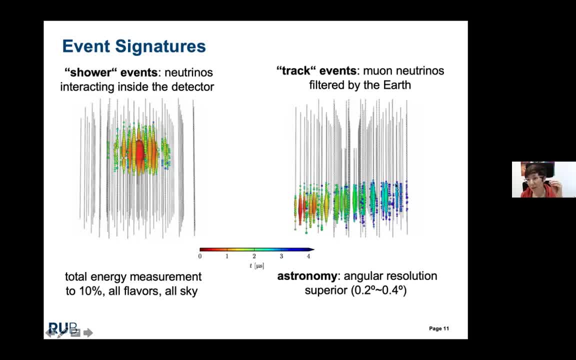 track events. You get that if you have a muon neutrino, that is, a charged current interaction. so you produce a muon and this muon can travel a long way through the eye, several kilometers, depending on its energy. And you can clearly see from the different arrival times on the 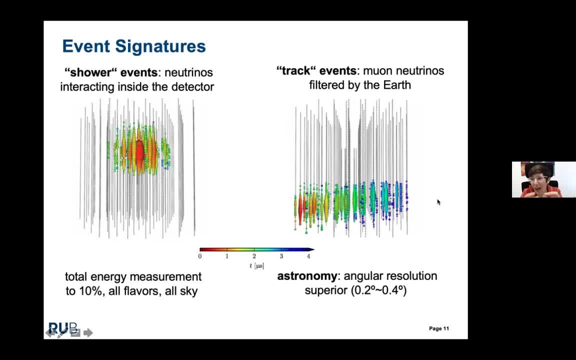 optical modules that we can even by eye. you can construct the direction of the incoming particle here. So we will mainly focus on those events, because we want to use them to astronomy and to point somewhere. Yeah, so with IceCube we actually succeeded for the first time to measure a diffuse flux. 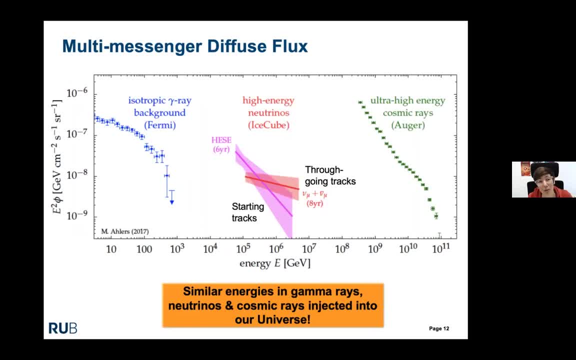 of high energy neutrinos. That happened already in 2013.. Here I show you this diffuse flux. So you have the energy here and the flux scaled with the e-square, and it's just two different action channels that give you the two different lines. here And in this plot, I compare the diffuse 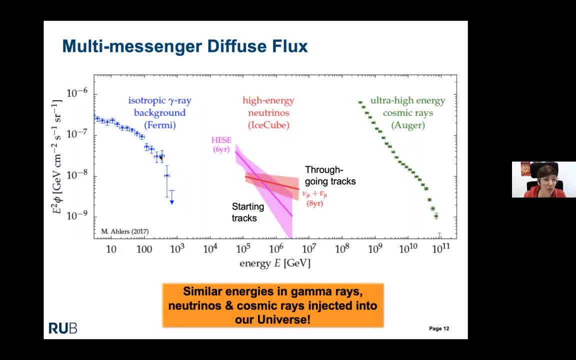 neutrino flux to the diffuse gamma-ray flux measured by Fermi, shown here in blue, and the cosmic-ray flux measured by Auger, And in this representation you see that more or less the fluxes are on the same level, telling us that actually similar energies are injected into the 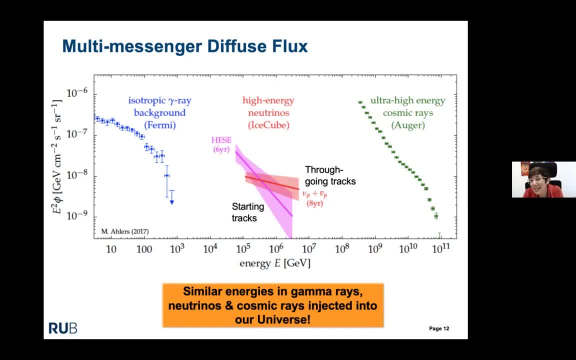 universe in those different messengers. That indicates that they all come from the same source. but we don't really know that yet Because after detecting a diffuse flux, obviously the next step is to figure out where those astrophysical neutrinos are actually coming from. 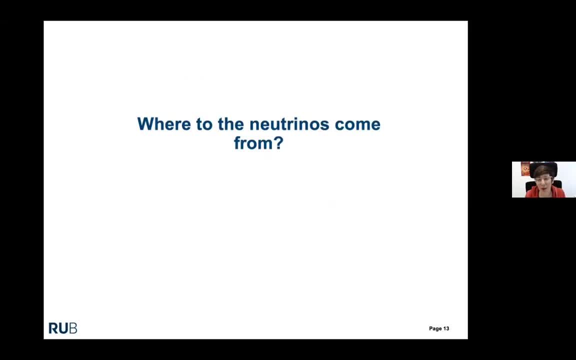 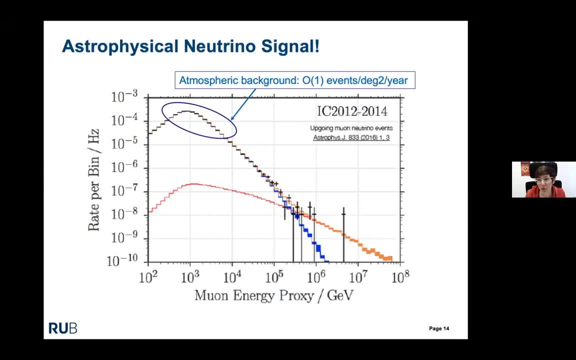 To figure this out is actually tricky, because we don't only see the astrophysical neutrinos, we also see a bunch of background in our detector that's coming from the atmosphere, Cosmic-ray rays hitting the atmosphere, and then you produce air showers, and in those you also 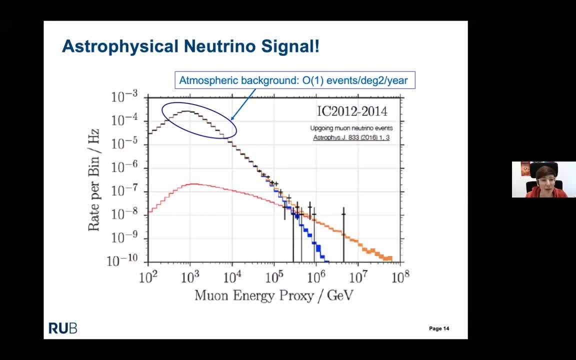 produce neutrinos and muons that would also enter the detector And I think this is nicely illustrated in this histogram just showing the event rate as a function of the muon energy proxy. And in black you see the measured data and in blue is what we expect from atmospheric background. 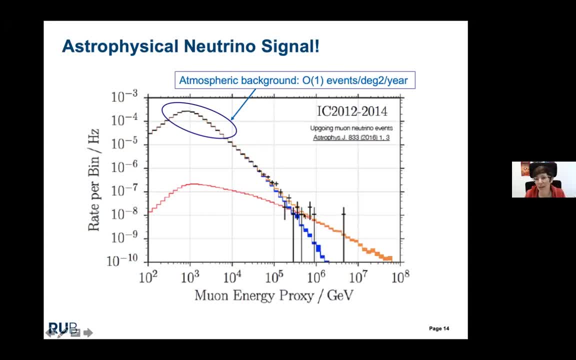 So you can clearly see at high energies that there is some excess, and this is produced by that diffuse flux That I just showed you. And now you can somehow model the signal, neutrinos, and here we can really measure them. but at low energies it's not really clear. so you can try to. 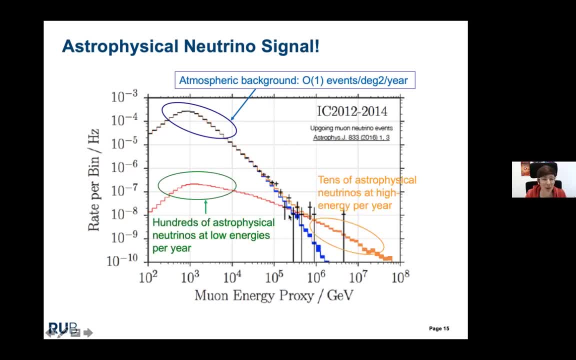 somehow extend the flux also to lower energies. So we expect that there's probably hundreds of astrophysical neutrinos at low energies per year. however, those are buried in a huge atmospheric background of roughly one event per square degree per year. However, at highest energies, 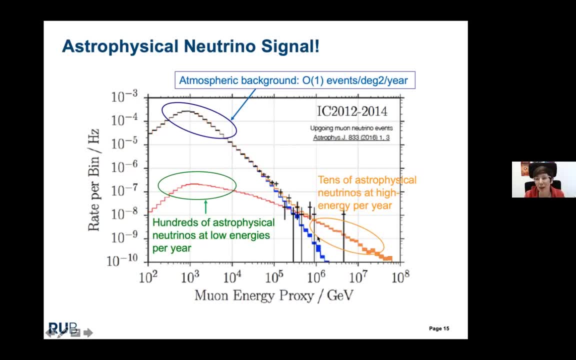 actually we get. if we find an event there, we are quite certain that it's an astrophysical event, but at the same time our statistics are very low. so we have only tens of astrophysical neutrinos at high energies per year. In my talk I will focus on actually this high energy part. 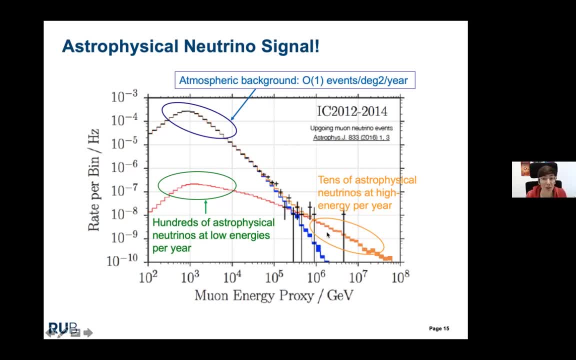 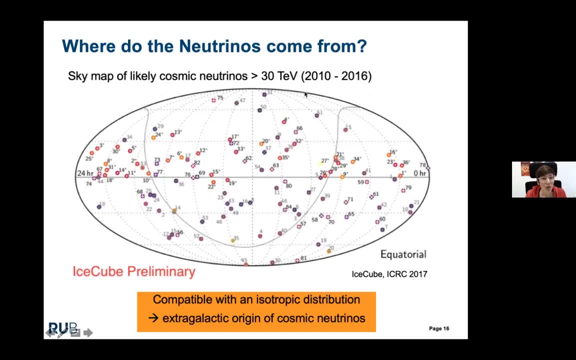 to try to figure out what are actually the sources of those high energy neutrinos. So the first thing we could do is to make a sky map of those high energy neutrinos. so those are now all the neutrinos that reach energies larger than 30 TeV. 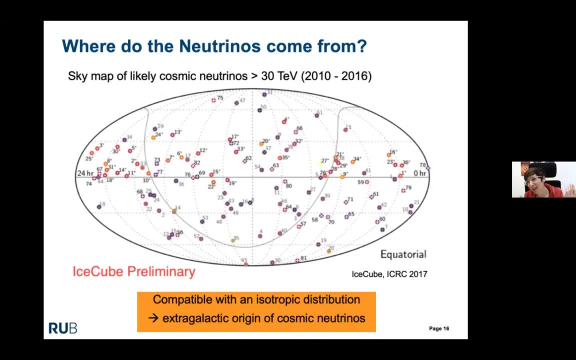 With that energy threshold, roughly half of the events are astrophysical and half of the events are still atmospheric background events. Yeah, now you can look at the distribution. This is an equatorial coordinates. The galactic plane would be this gray line here. So what you don't? 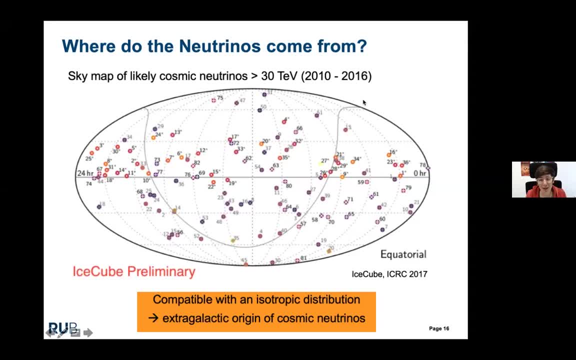 see in this plot is an obvious clustering of events along the galactic plane. that indicates that most of the flux has to be of extragalactic origin. What you also don't see is some obvious strong clusters somewhere in the sky, so that tells us that we don't have just a few. very 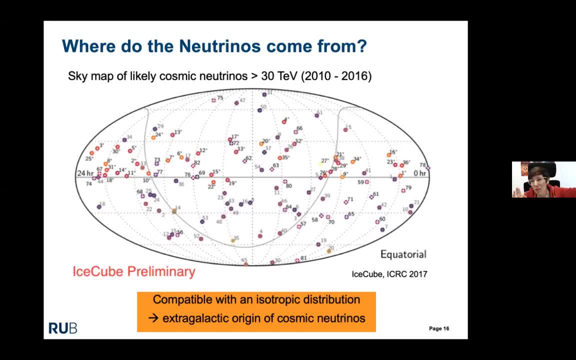 bright neutrino sources, but we're probably dealing with a lot of dim neutrino sources in the extragalactic sky. So how can we now try to figure out where those neutrinos are coming from? My talk is about multi-messengers, so we have to combine. 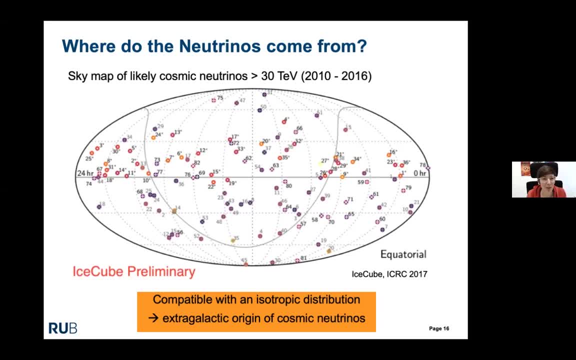 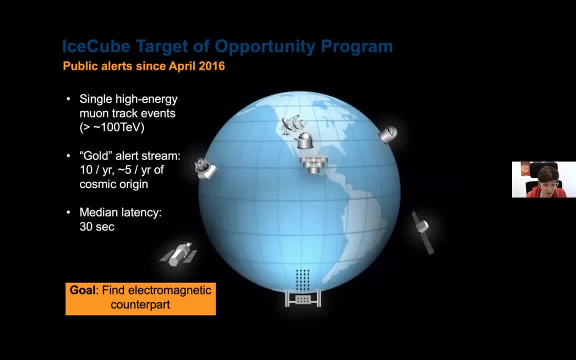 now the neutrinos with a different messenger and they will be photons. So we have set up a target of opportunity program to increase our sensitivity to identify the sources of the neutrinos, especially transient and variable sources, And the idea is that with IceCube at the South Pole, we can detect neutrinos in real time and reconstruct their direction. 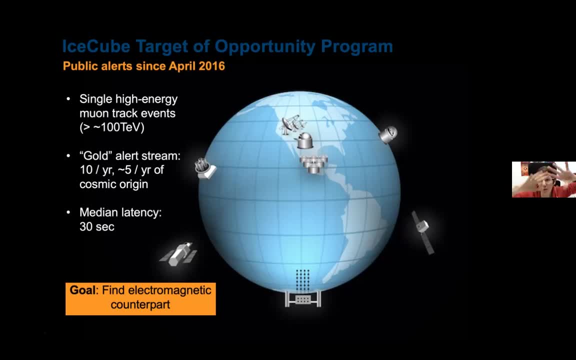 and then broadcast this information immediately to a network of telescopes around the world, And then those telescopes would immediately, or as soon as possible, slew and observe the direction of the hydrogen neutrino and then hopefully find an electromagnetic counterpart in the sky. And we can do this whole alert forwarding. 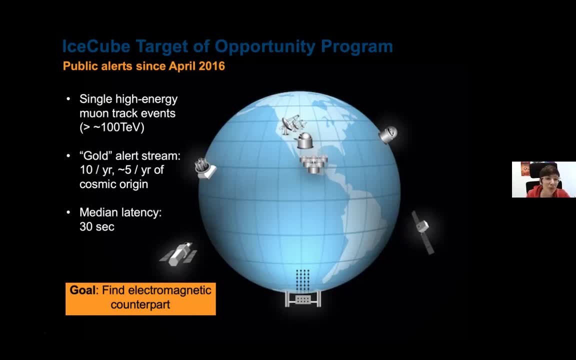 with a median latency of 30 seconds And at the moment, to the public, we sent out a bold alert stream. This consists of those high-energy track events that I showed you, because obviously we want some decent angular resolution And we apply an energy threshold more or less at 100 TeV. 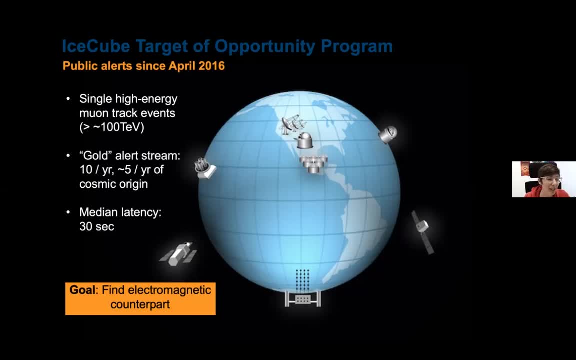 That gives us this gold stream, our best events, roughly 10 per year, And we expect five of them to be of astrophysical origin. And there's still a contamination- 50%- from atmospheric background. So the program started in April 2016.. And I will show you now a few interesting candidates that we 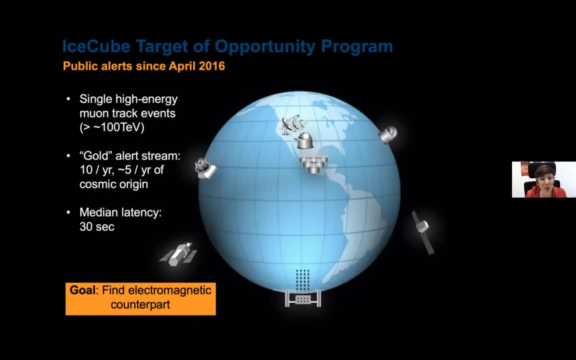 have identified. So the program started in April 2016.. And I will show you now a few interesting candidates that we have identified. The most famous one that probably most of you have seen was a high-energy neutrino that was detected in 2017, in September. 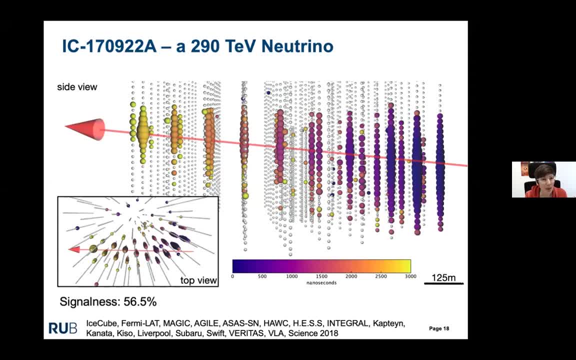 It had an energy of almost 300 TeV And here you see the event display. So it's a nice track event. It had a signalness of 56%. That means the probability that this is an atmospheric event, a background event, is still 45%, So by itself it's a very good signal. 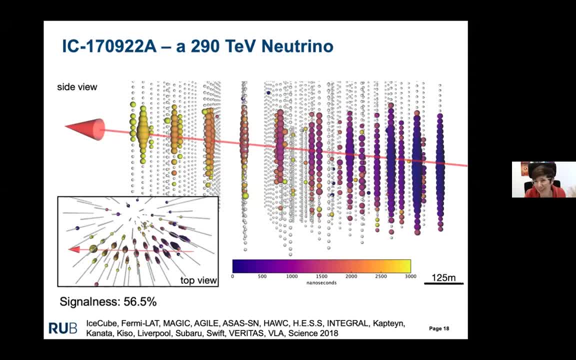 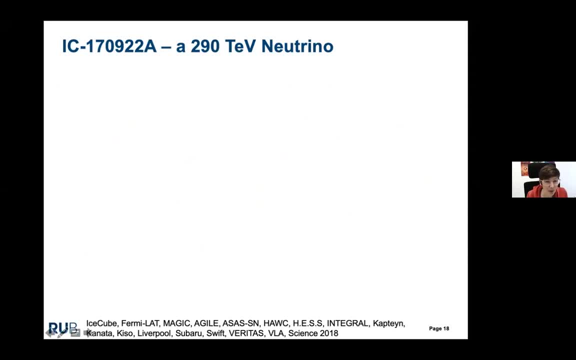 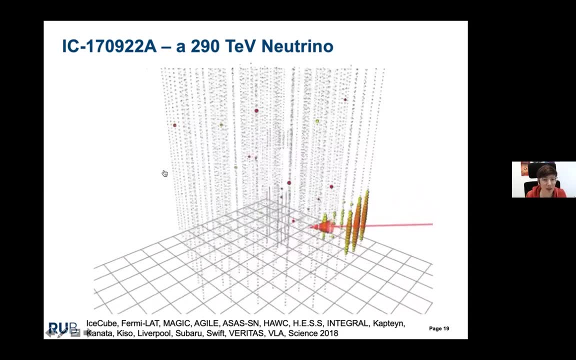 So by itself the event is not super interesting because we still don't know is it the signal or a background event? And I will show you a small. So yeah, it's an animation. You see, there's a little bit of noise in the detector. Now the 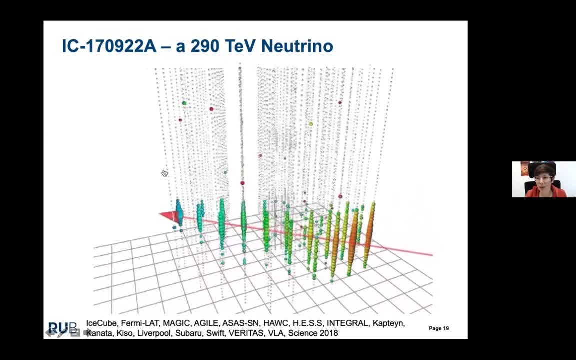 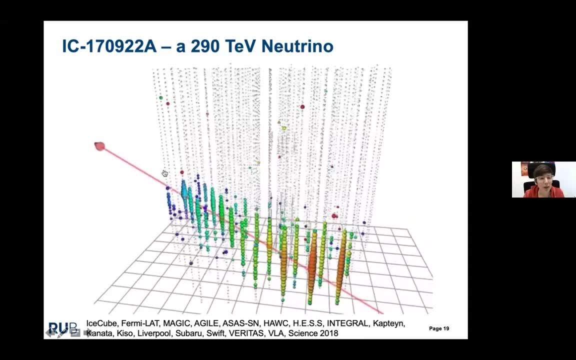 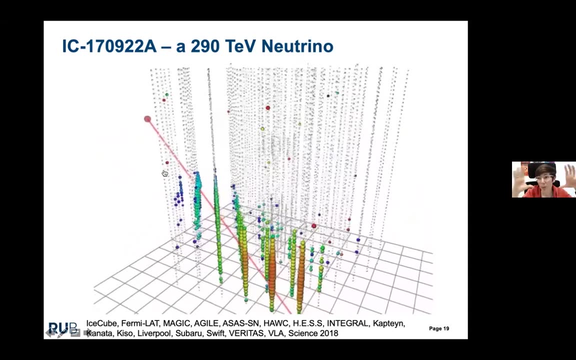 muon enters the detector and you can nicely see how it leaves this trail of cheering of light And it gives us now a nice lever arm to reconstruct the direction case, the, the area that covers the 90 percent probability of having the true direction in there. 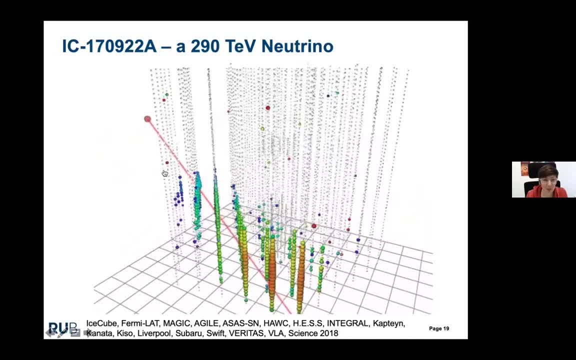 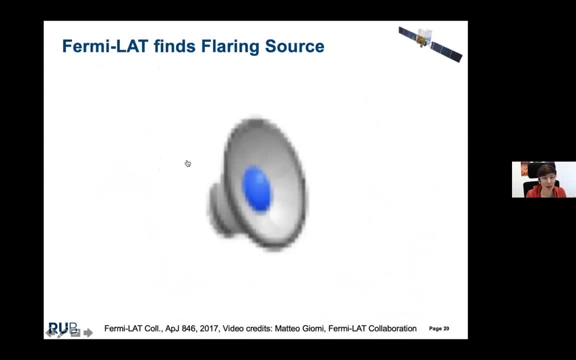 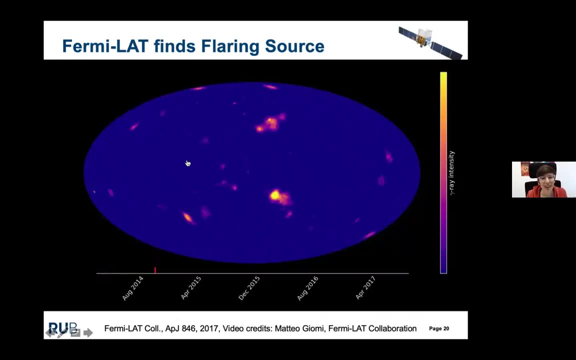 was one square degree in the sky. Yeah, as I said, by itself the event is not very interesting, but if we now take it together with gamma ray data, it actually becomes very interesting. So this movie here shows the sky in GV energies as seen by Fermi. Each image is one week of data subtracted. 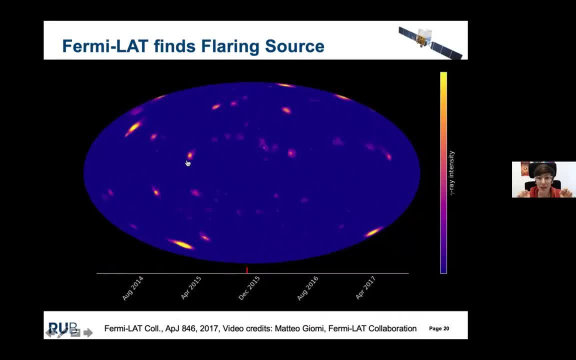 from the average sky map. So everything you see here is just little variations or strong variations in the sky. You see, there is a lot going on in the gamma ray sky. If you look carefully, you can even see the sun moving through, And now in 2016, we started our neutrino program and you see the 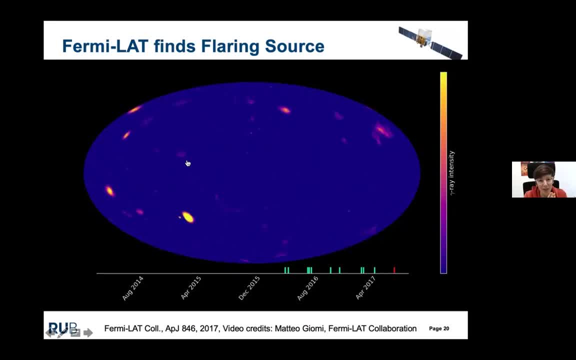 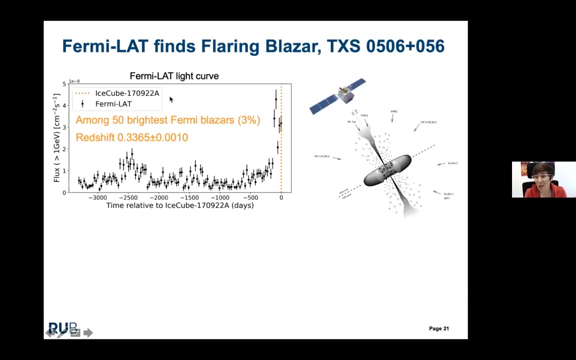 neutrinos popping up in the sky And the interesting one happened in September 2017, and now we zoom in, you see that the neutrino is right on top of one of those fluctuations in the sky. So we took a closer look with Fermi, and the source that produced this flare is actually an already known bright gamma ray blazer. 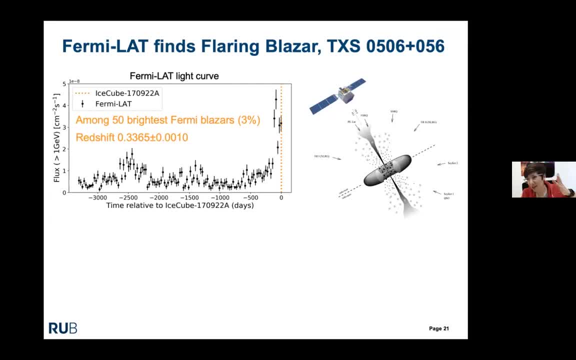 t-cell. So a blazer is an active galaxy where our line of sight is aligned with the blazer jet And those sources dominate the gamma ray sky, the extragalactic gamma ray sky, And you see a light curve here in gamma rays of the source in days relative to the arrival. 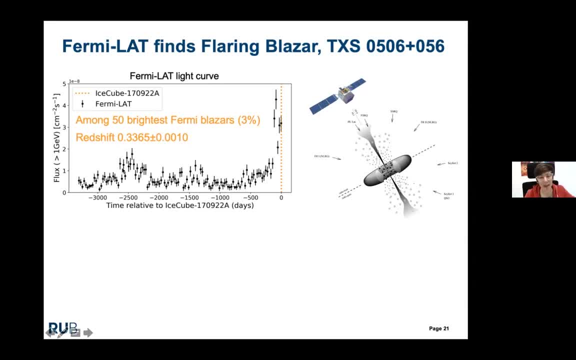 of the neutrino and you see that, yeah, it's almost 10 years of data that we have from the, from the Fermi survey, And there was some variability in the past, but really this largest flare of the source happened exactly when the neutrino arrived. This blazer is among the 50 brightest. 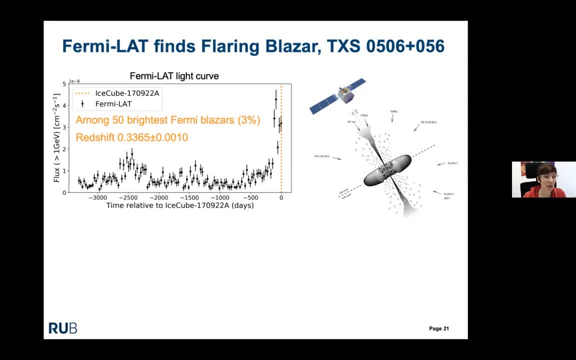 blazers in the Fermi catalog that brings it among the top three percent. Initially the redshift was unknown but after we found the neutrino from the direction of the blazer there was a campaign measuring the redshift and it was found at 1.3. 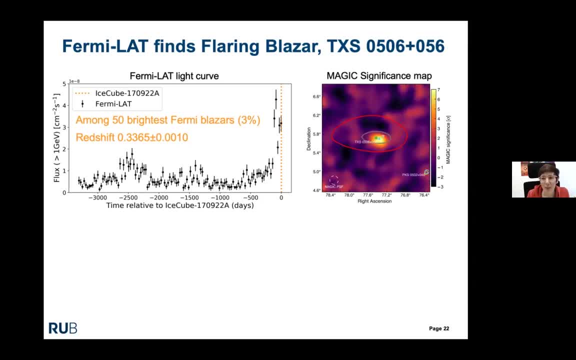 In addition, this source was then also for the first time first time detected in very high energy gamma rays by the magic telescope. We see the significance map here. the source is right here and this is the best-fit neutrino position, and you see the 50. 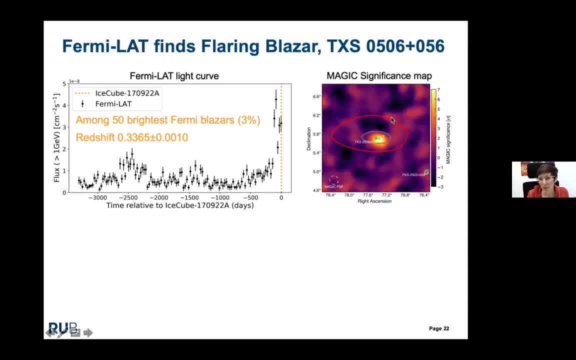 and the 90 percent uncertainty region of the neutrino. So really the source was nicely aligned with our best-fit position. Yeah, now you have to ask yourself, how likely do we find something just by chance? right, We just randomly look somewhere in the sky? what's the chance to find the flaring? 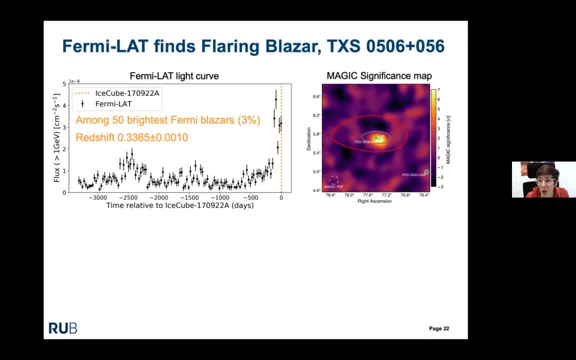 laser in that direction And it's actually pretty small. We did the calculation and we also took account for trials, because we have done this experience several times. We also looked at archival data. so, including all this, we find a three sigma significance of this association. 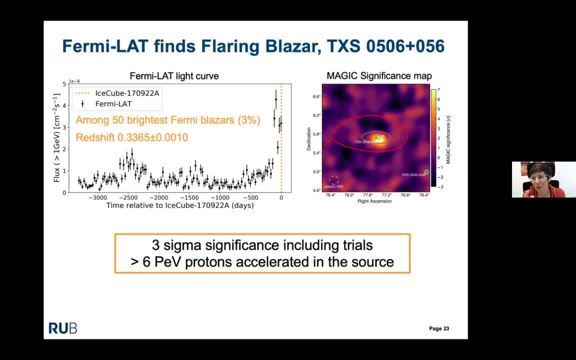 So that's maybe not convincing a particle physicist who was looking for five sigma accesses, but for us this was actually at that time the first and only three sigma association with the source that we have found, so we're quite excited about this association. So if we now believe the neutrino was really 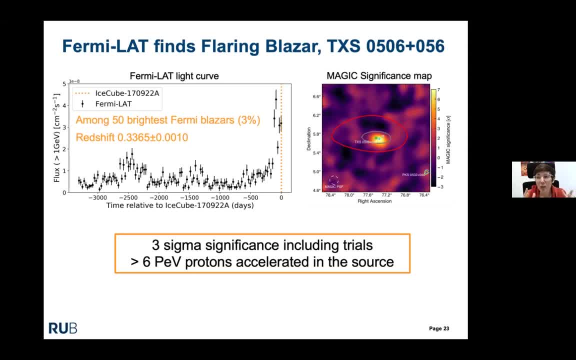 produced in that source. that tells us that there has to be high energy protons accelerated in the source at least to fuel PEV energies to produce the neutrino at the 300 TeV. So now I talked a lot about the gamma rays we've seen from the source, but there's 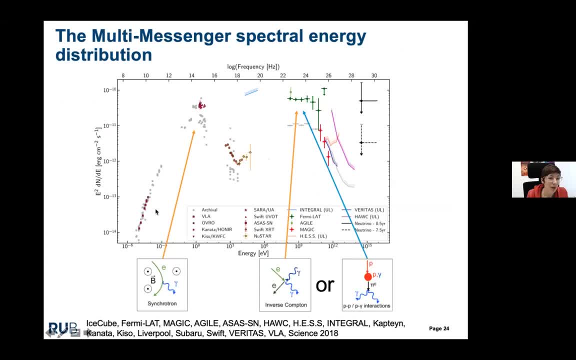 actually much more data from the source, ranging from radio to optical, to x-ray to gamma rays here. so this is the spectral energy distribution of the source, And now obviously we want to know what is producing this emission from the source. We are pretty sure that the low energy pump is produced. 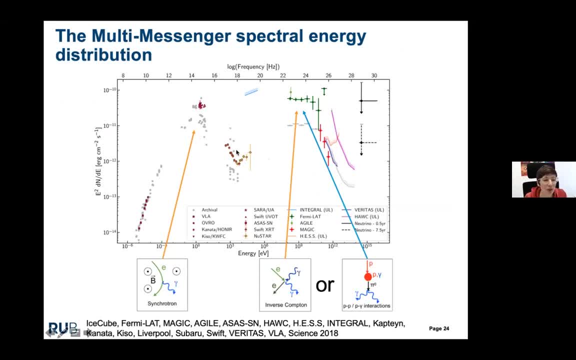 by electrons and neutrons. So we're pretty sure that the low energy pump is produced by electrons being bent in the magnetic field in the source and producing synchrotron radiation. For the second bump it's not so clear what is causing the radiation. It could either be: 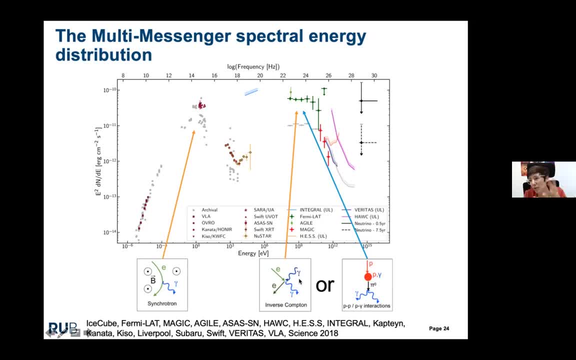 for example, the same population of electrons that is upscattering, for example, the synchrotron protons, to high energies in inverse quantum scattering processes. There would be a leptonic model, or it could be high energy protons in the source interacting, for example, with photons. 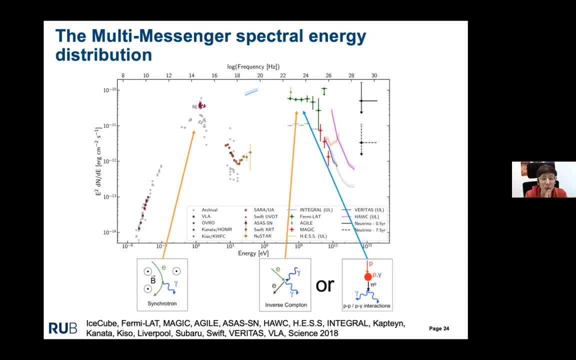 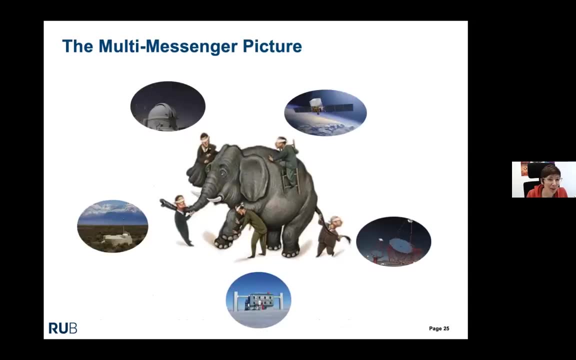 and producing pi zeros. that would then decay, Producing gamma rays. That would be a hadronic model. And if we believe that the neutrino came from the source, then we know there have to be some hadrons in the source. So if we go back to our multi-messenger picture from the beginning, 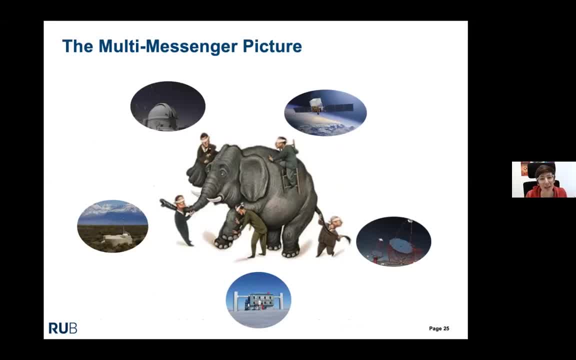 then maybe now you realize there is actually something missing in that picture where I saw I showed you all the observatories and what is missing here is the theory. So now we have to give all our data to the source and then we have to go back to the source. So if we go back to the source, 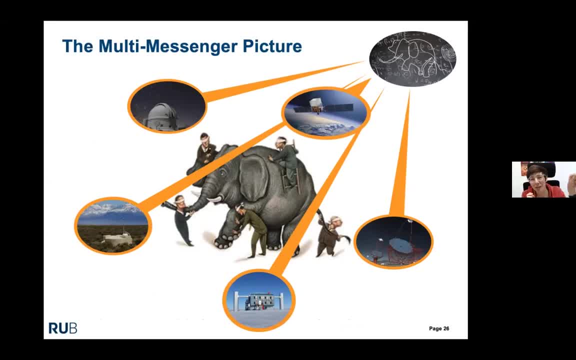 we have to go back to the theorists that would then basically draw a picture of the elephant or tell us what is actually going on in the source, And many theory groups have actually modeled this source, And I'm just showing one example here, but I think most of the groups 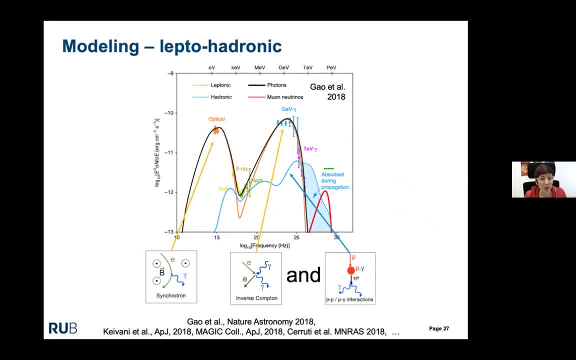 came to the same conclusion for this high energy neutrino arriving in 2017.. Again, you see the spectral energy distribution with all the data collected here, And in this model they actually chose a combination of electronic and hadronic processes, So you have relevant. 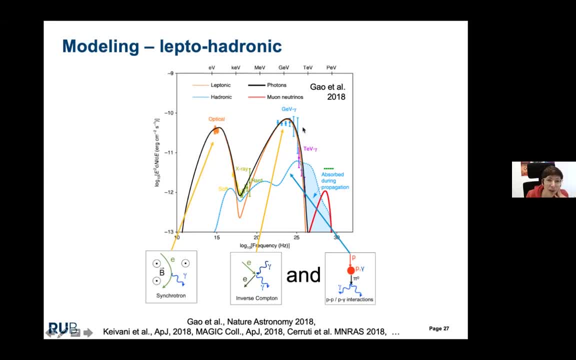 N-protons in the source, and in orange you see the electronic part of the model and in blue you see the hadronic part. And what is actually interesting here is that most of the gamma rays that we see, especially the GEV gamma rays measured by Fermi, are actually dominated by the lepton model and not 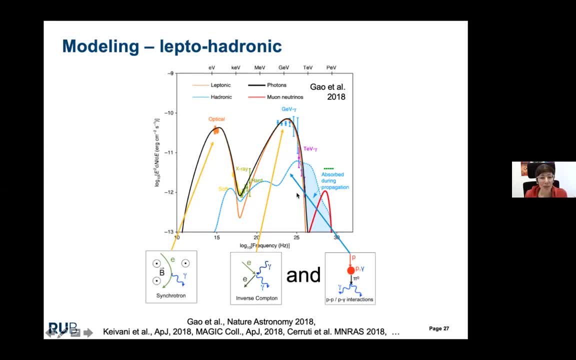 the hadronic model. So where you can really see the hadronic model is here in the X-ray regime and then also at very high energy gamma rays, And this model would then also produce a decent amount of neutrinos that could explain this one high-energy neutrino that we have detected. So now the question is: did we solve? 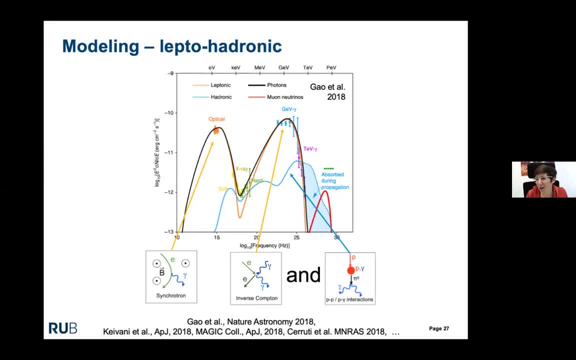 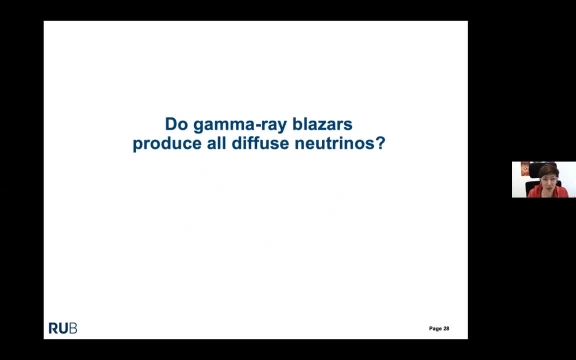 the puzzle. Do we actually now understand where all the neutrinos are coming from? So do all gamma ray blazers produce neutrinos, and is the flux sufficient to explain the diffuse neutrino flux? And the answer is actually no, because if we now look at the population of gamma, 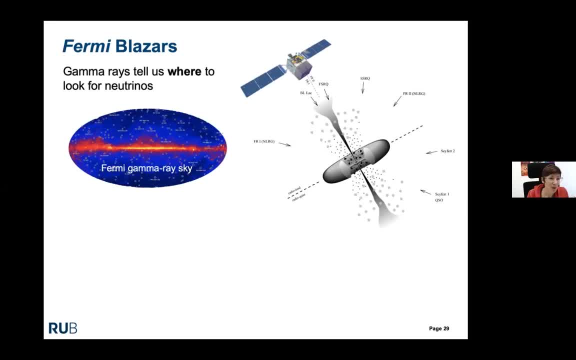 ray blazers seen by Fermi. so this is the Fermi sky map and all those dots here at high latitude. almost all of them are actually blazers. And what the IceCube collaboration has done here? they took a catalogue of those gamma ray blazers and looked for an excess of neutrinos from those directions. 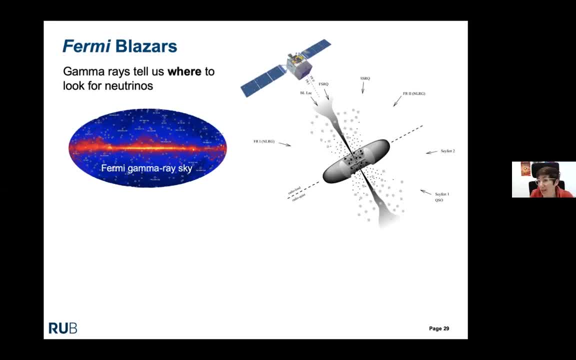 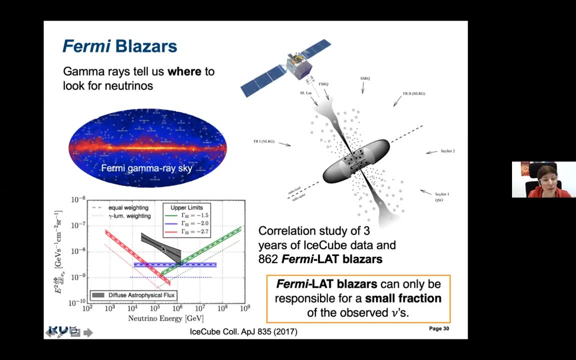 combined in the sky And no excess was found. That allows us to now set an upper limit on the contribution of those gamma ray blazers to the diffuse neutrino flux, And this is seen here. so in black again is the measurement: the diffuse neutrino flux. And now, if we, in the most naive 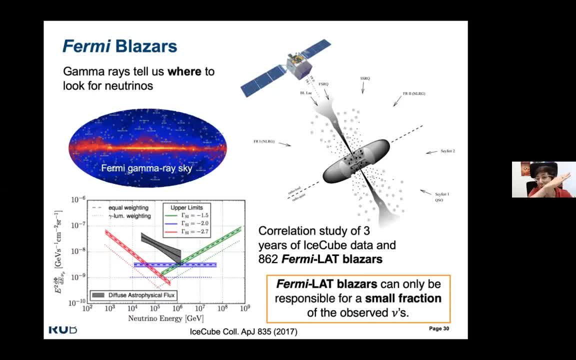 assumption: assume that the neutrino spectrum producing the neutrinos would follow exactly the same shape as the diffuse flux. then you get this red line as an upper limit And you see that you can really only produce a few percent of the diffuse flux by blazers. However, you can also assume that 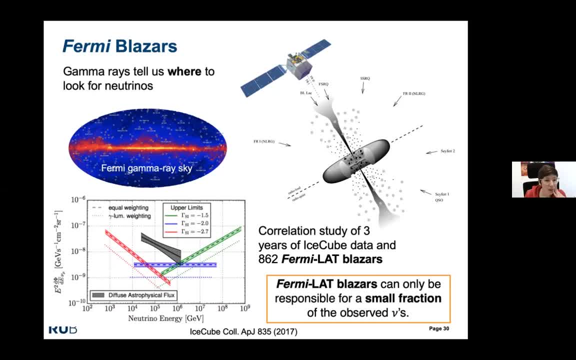 maybe the spectrum is different and it's actually harder. so there would be this blue or green case And in that case you can actually produce quite a large fraction of the diffuse flux, but only at high energies, And you miss the low energy. You miss the low. 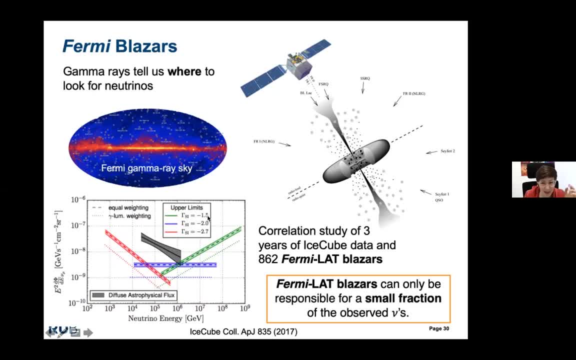 energy part. So the conclusion here is that Fermi blazers can only produce a small fraction of the observed neutrinos, But, depending on the assumption you make in your analysis, actually they could produce a large flux at high energies without explaining them. the low energy part. 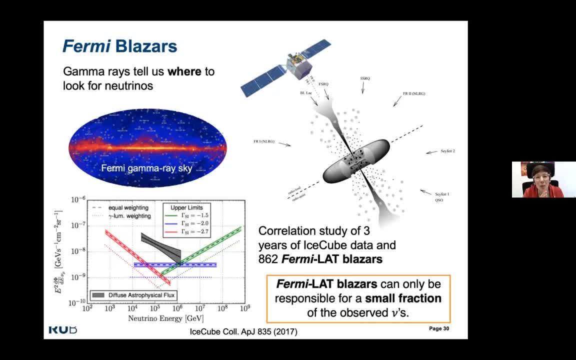 So that tells us that probably there's more than more neutrino source class, And I just drew this here by hand. So if we imagine that the blazers produce the high energy part, then there has to be some other source class producing the the low energy part. And that wouldn't be such a surprise, because it's also what we see in the 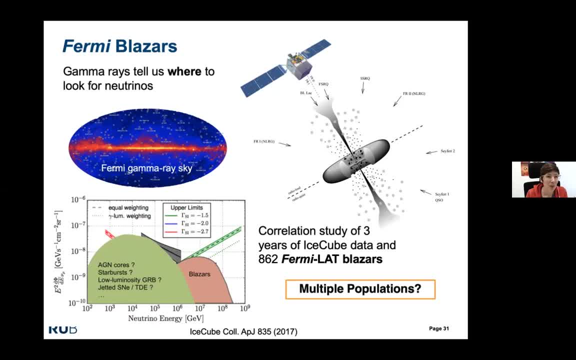 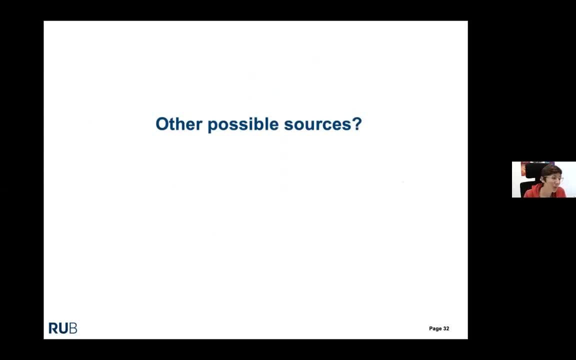 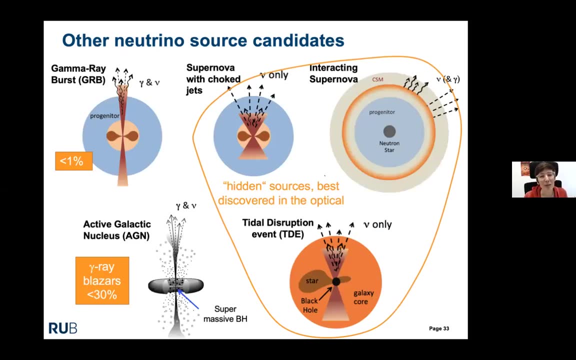 electromagnetic sky, right, So yeah, then the obvious next question is: yeah, what are the other sources that produce the rest of the neutrinos? And there's a bunch of candidates just showing a selection here of probably some of the most promising candidates. So we talked about 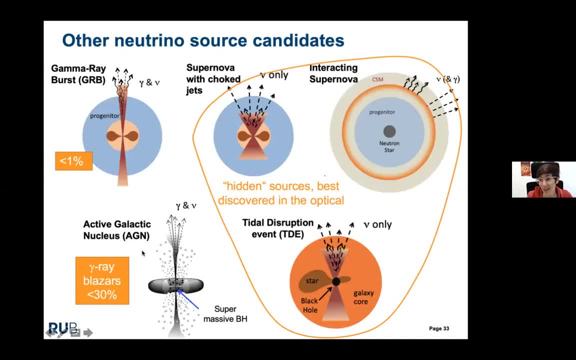 blazers. Those produce less than 30% of the diffuse flux, But those are the blazers right, So it could also be maybe other types of AGM where we do not look along the jet. Another promising candidate: Montgomery bursts. 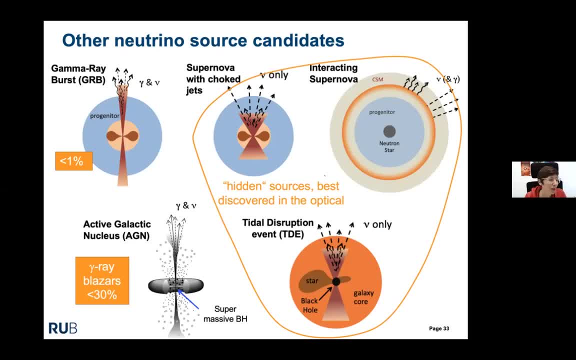 I think when I skipped started, people were most excited about Montgomery bursts as potentially neutrino sources, And here we did a similar stacking analysis where we used a catalog of Montgomery bursts and searched for neutrinos at the time of the prompt emission, which is a very sensitive search because you can reduce the atmospheric background a lot. 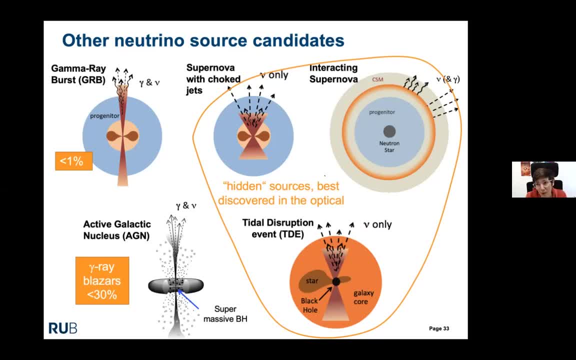 You only look at a very short time window and no excess was found. So Montgomery bursts actually very much disfavored as the prime source of the diffuse neutrino flux. They can of course still produce neutrinos, it's just not a lot of the flux that we're seeing. 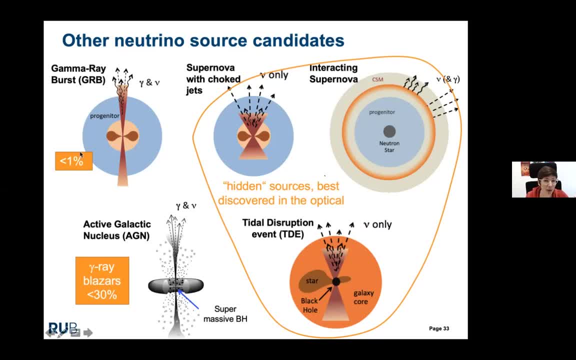 so it would be less than one percent of the diffuse flux. And then we have a bunch of other sources I'm showing here. So maybe gamma-ray bursts are just the tip of the iceberg, but they could be a much larger population of failed gamma-ray bursts or short jet supernovae, where 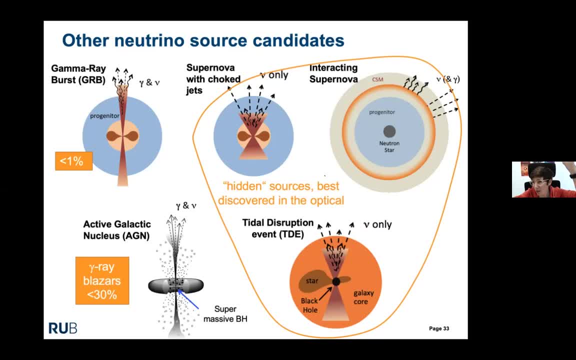 you also produce a jet. but this jet wouldn't be able to penetrate the surface of the star. it would get stuck in the surface of the star, absorbing all the gamma rays. but the neutrinos of course can still escape. And, yeah, you wouldn't see then the gamma rays, but you could still see. 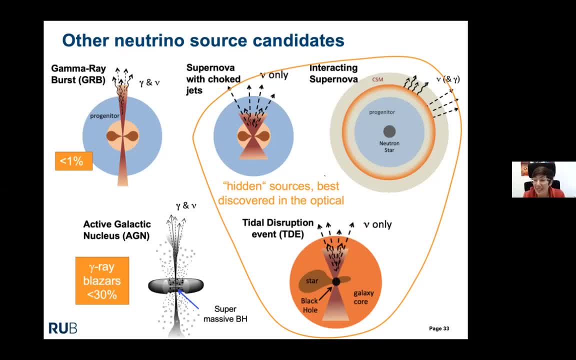 a supernova counterpart. They could also be interacting supernova, that supernova exploding in a very dense circumstantial medium and then the ejector would interact with the dense medium, also producing high energy neutrinos. So that is a bit similar to supernova remnants. 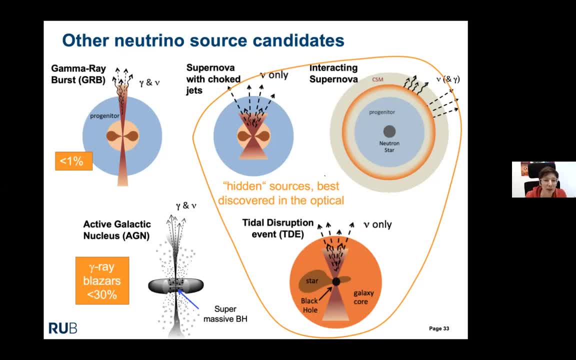 but on short term timescale And another source candidate- tidal disruption event. also here you have a supermassive black hole and a star getting too close to that being ripped apart, And that's something I want to focus on now, and this is a. 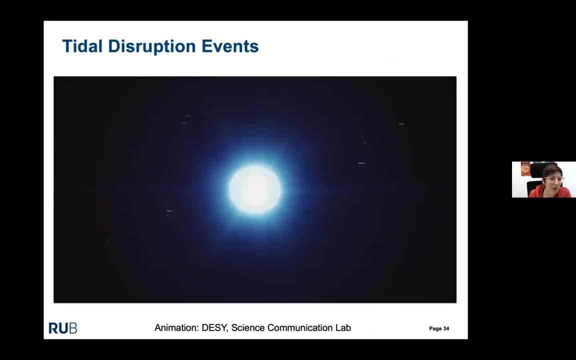 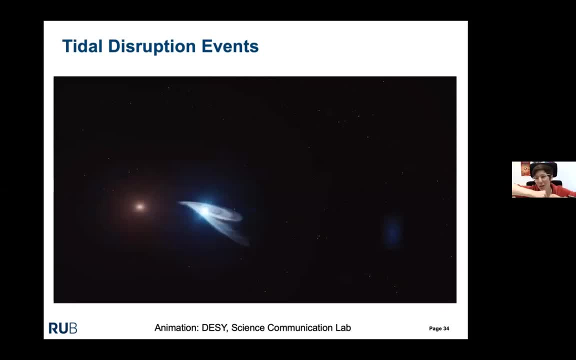 nice video illustrating what happens. So we have the black hole and the stars getting too close to the black hole. You see the tidal forces kind of struggling to get close to the black hole. So that's something I want to focus on now: stretching the star and eventually ripping it apart and part of the debris is pushed. 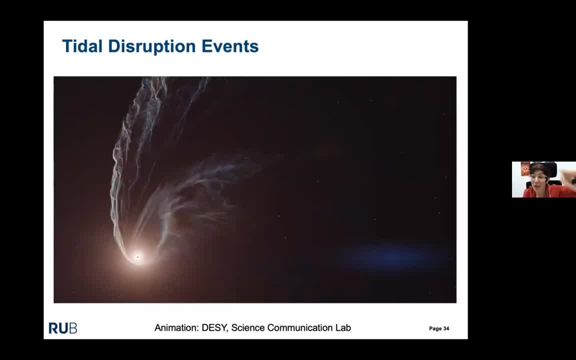 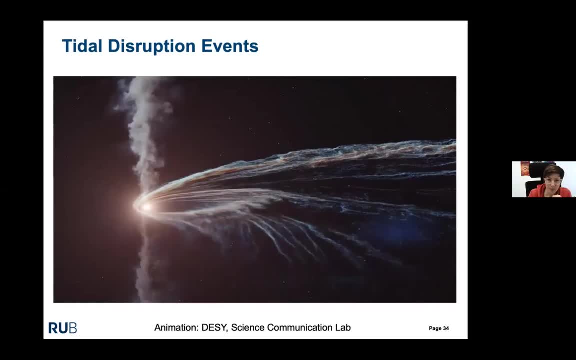 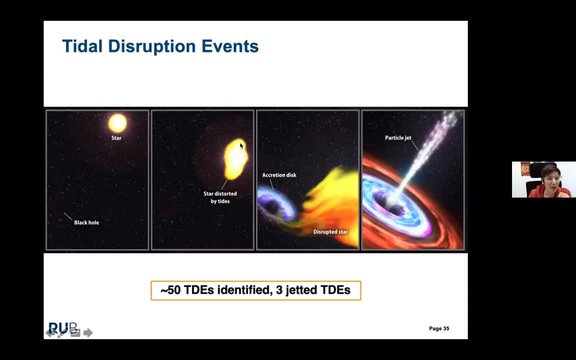 away into space and some of it will be accreted onto the black hole and in some cases you can also produce a relativistic jet. And this is the same thing again in pictures. here you have the star approaching the black hole. it gets distorted and eventually ripped apart and has been accreted, and only in some. 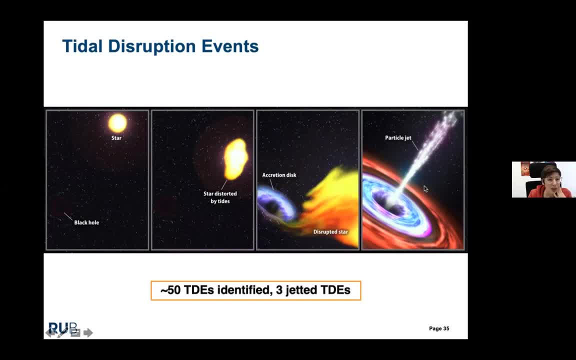 cases a relativistic particle jet is produced. So TDEs are relatively new objects. I would call them because only now, with the modern optical survey instruments, we actually managed to find a larger sample of those sources. So right now we have maybe 50 to 100 candidates for TDEs. only three of them have strong indication. 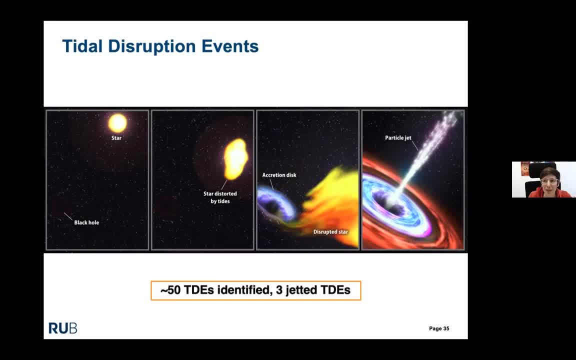 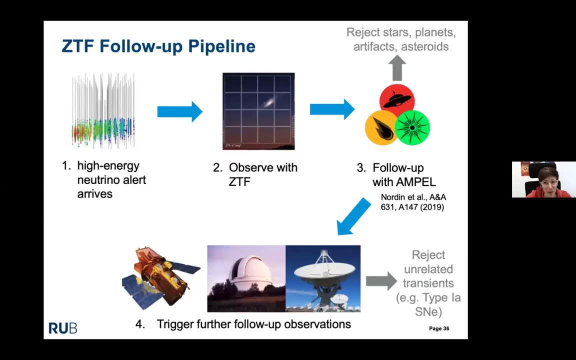 of a relativistic jet. Yeah, so how can we? how can we now search for neutrinos from those objects? They're actually best discovered in the optical. so we have an optical follow-up program, implemented where with the Zwicky transient facility, and I'll show you the instrument in a bit. 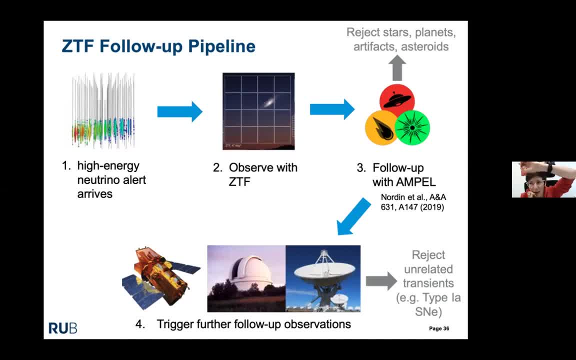 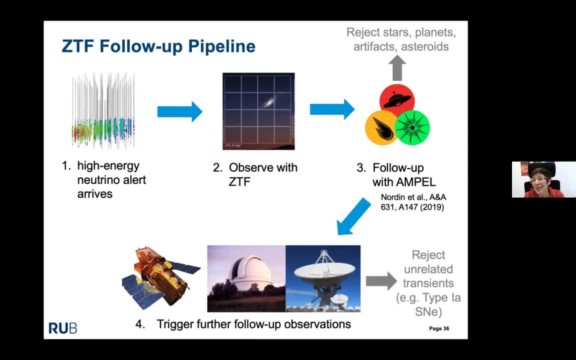 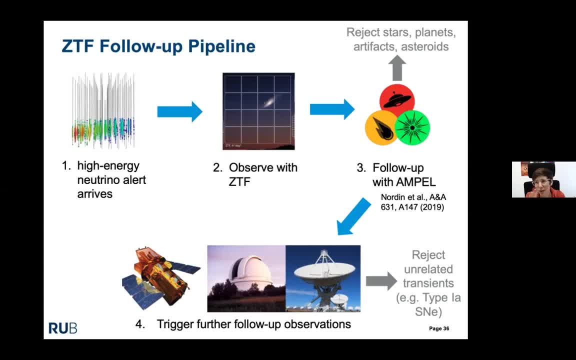 are not interesting: Stars, planets, artifacts from the image subtraction, asteroids and so on- And then we usually are left over with a handful of potentially interesting candidates, dates, and then we schedule additional follow-up in different wavelengths over different spectroscopy to really classify the sources that we have found in our follow-up and this additional step allows. 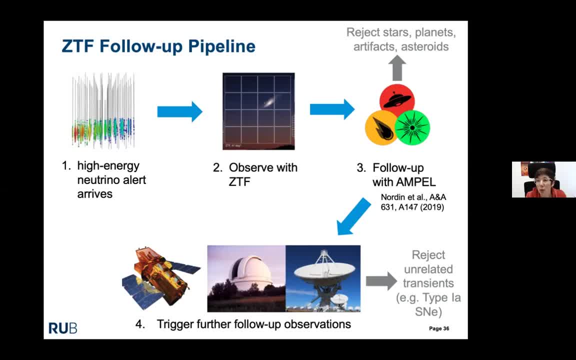 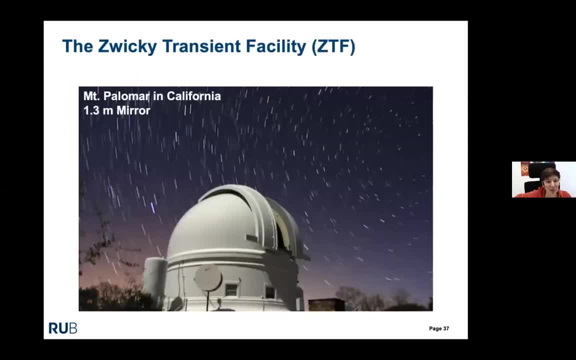 us to reject unrelated transients, for example type 1a supernova, that we believe have not produced high energy neutrinos. so this is a picture of the dome of this wiki. transient facility is an optical survey instrument located at mount paloma in california with a 0.3 meter mirror. this 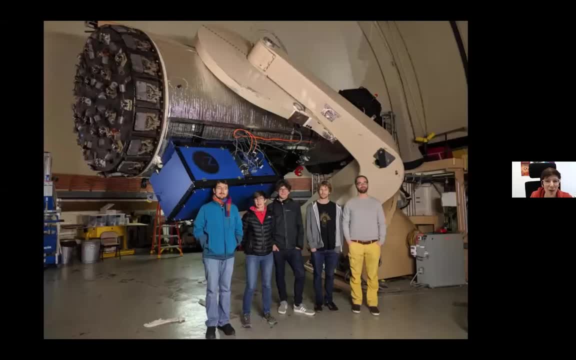 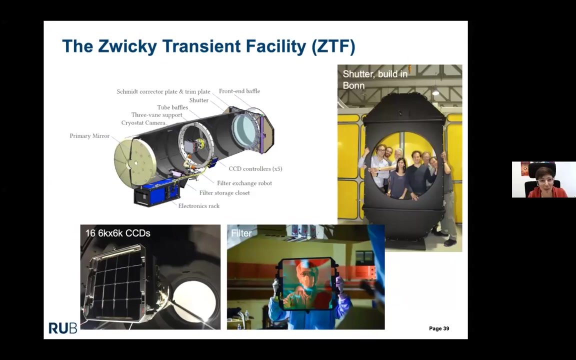 is how it looks from from the inside. so the, the mount and everything is actually old from the 60s, but everything inside the tube was was replaced for the wiki transient um facility and actually the. the hard piece of the instrument is the camera that is located here inside um the tube. 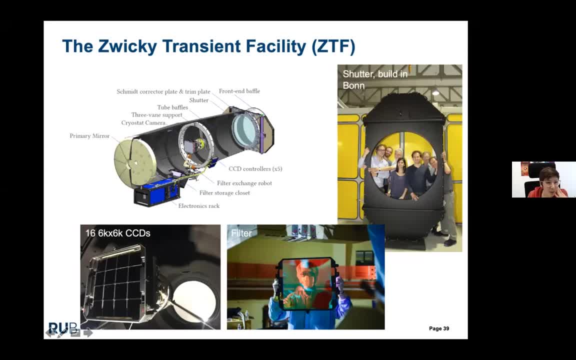 and to get an impression of the size, here's a picture of the camera and, for comparison, this is the filter that has the same size as the camera. here, with the human in the picture, you see that it's quite, quite a big camera. the other thing that's special about this instrument is the shutter. 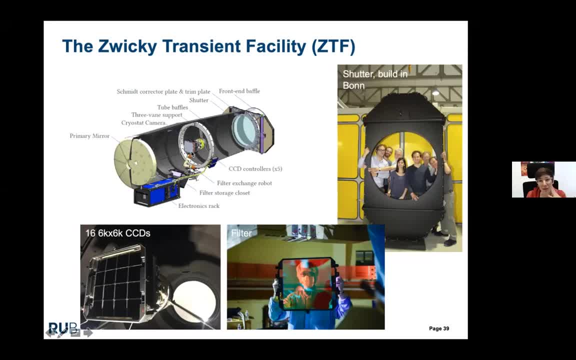 there was no space to have the shutter inside in front of the camera. it had to be put outside and therefore it had to be huge. and it was actually built in bond in germany and then tested at daisy. so this is the picture at daisy of this gigantic, of this gigantic. 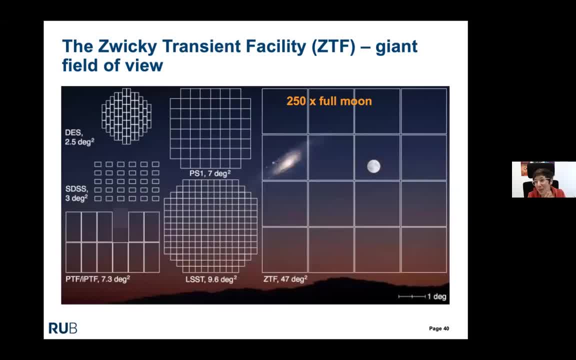 shutter, and so the large camera allows the instrument to have a giant view. actually, with one single pointing we can cover 47 square degrees of the sky and- and this is actually to scale you compared to other optical instruments- and yeah, the adrenaline in the room is to scale. so 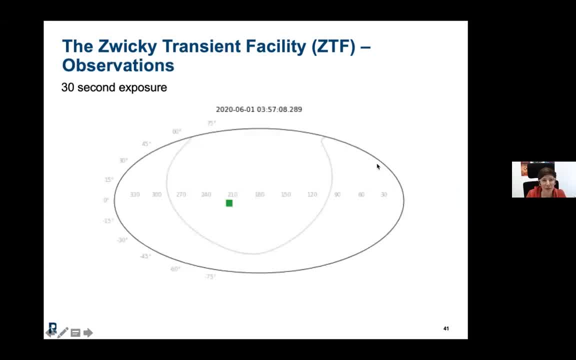 it's really a huge field of view, um, and and there's a bigger picture in front of the camera, that's, and therefore we can actually cover the entire visible northern sky almost every night. And this is a small animation here. Each little square shows one 30-second exposure. 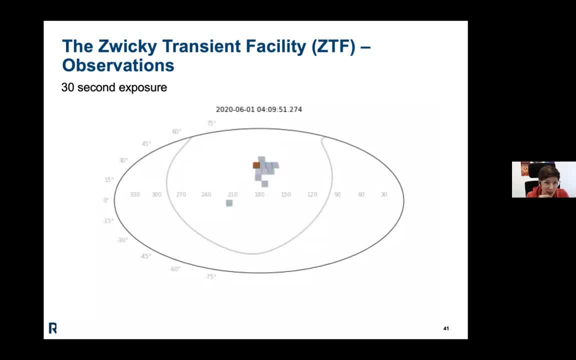 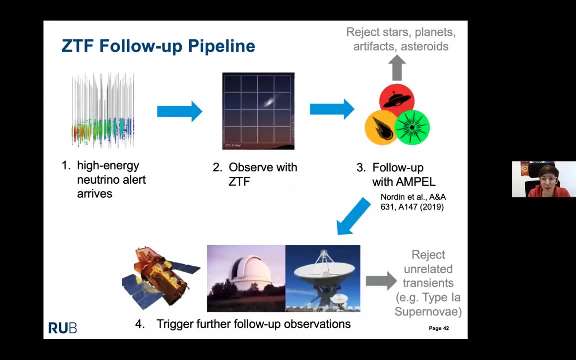 and this animation shows, I think, just four hours and how we cover the sky. So only this few hours we already covered quite a large part of the sky. I already showed you this. So yeah, once we see the neutrino, we point the telescope. 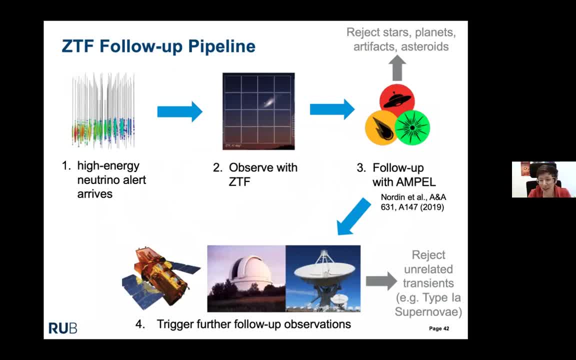 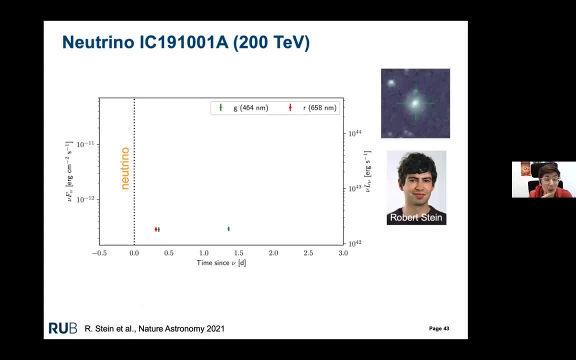 we have our algorithm identifying interesting candidates, and now I want to show you one of those candidates that we have identified. So we followed up a neutrino in 2019, and this work was led by a student at that time, Robert Stein. He graduated now and moved to. 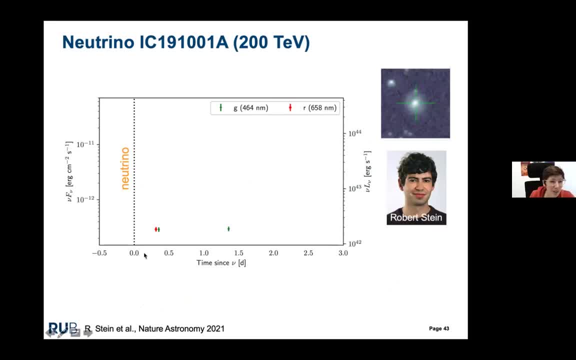 Caltech for postdoc. So the neutrino arrived here and then we took additional. We have the survey that covers the sky, normally at a three-day cadence, but thanks to our neutrino program we would then point the telescope, get data immediately. 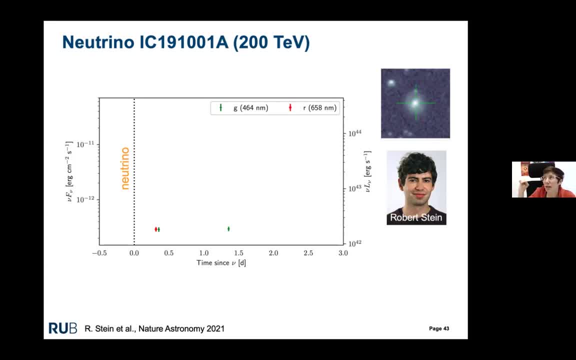 and we also take a deeper observation. So we take a 300-second exposure compared to the regular 30-second exposure that is applied in the survey. So we detected the source and this is a cutout of the image. So you see, there is some. 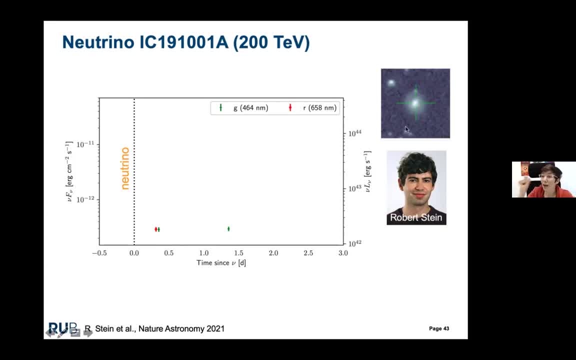 This blurry thing is a galaxy And the source was actually right-in-the-center-of-the-galaxy, which is already an argument against a supernova, for example. Yeah, so we took those to data points. And then the beauty about CTF is that they have this: 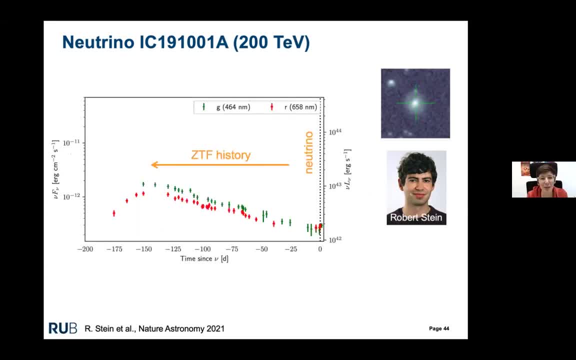 amazing archival data. So another response is: because it's very similar to something that. So we went back and looked in the archive and we found that there was actually quite an interesting source that peaked already 150 days ago And of course, that wasn't unnoticed by the ZTF team. 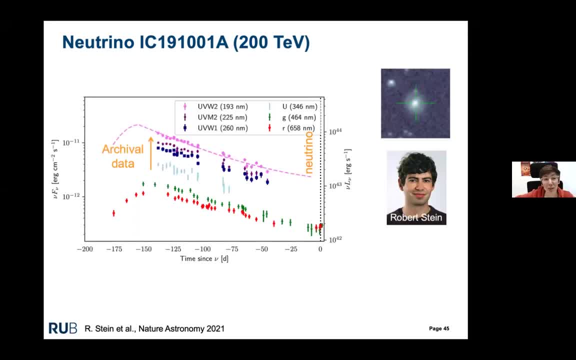 They had already identified that there was an interesting source. They triggered close to the peak, They triggered additional data in different wavelengths, which is shown here, And they measured the redshift to 0.05 and classified this event as a tidal disruption event. 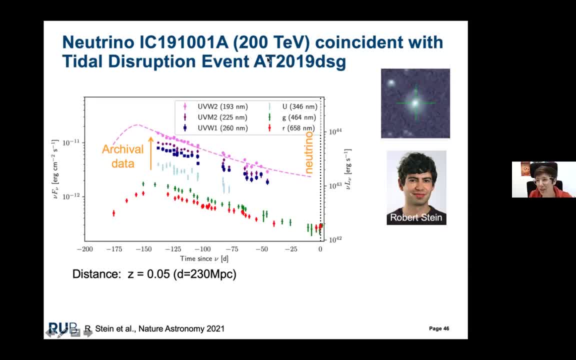 And it has the name AT2019-DSG, because those names are really hard to say and hard to remember. Because of that, the ZTF Black Hole group gives nicknames to all of their sources, And this one is called Brandstar. 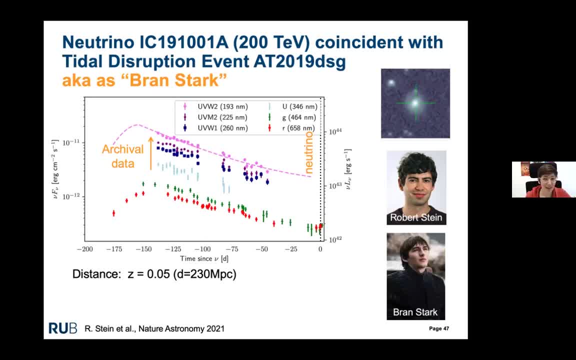 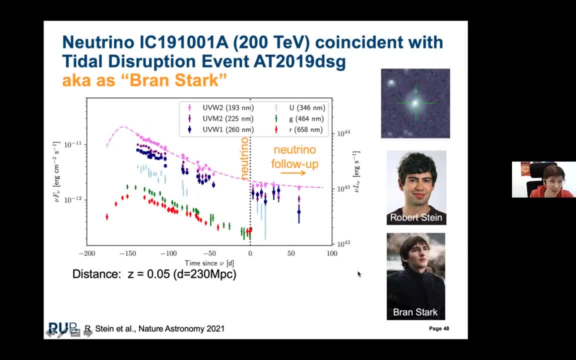 So they all have names. They're all named according to Game of Thrones characters, And this one is Brandstar. I thought that was funny because he looked a bit similar to Robert, And now, thanks to the optical for our program, we have the archival data. 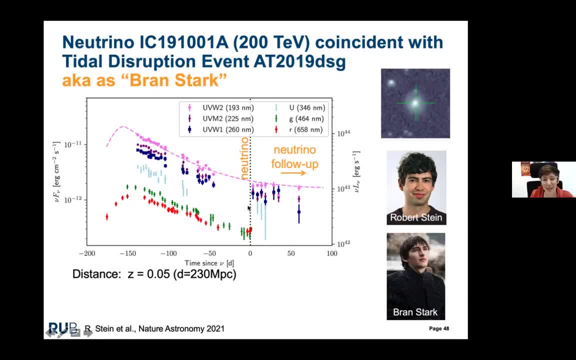 We also triggered more data in other wavelengths than you can see here. The next step would be to calculate how likely we see something like this just by tracking. So we have a chance And the chance of incident probability is small. It's just 0.2% to find a TBE incident with the neutrino. 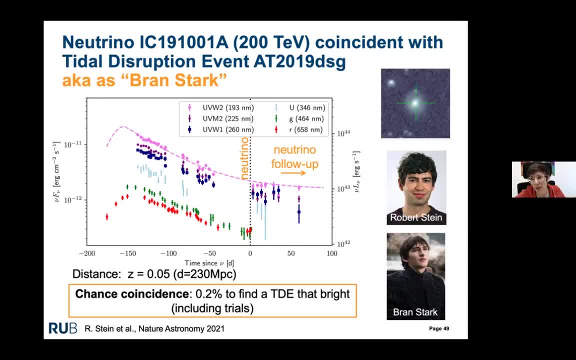 that has similar brightness. And this is also including trials, because we have performed a bunch of optical follow-ups already before, So this is also at 3 sigma level. What we thought was puzzling is that the neutrino arrives 150 days after the peak of the source. 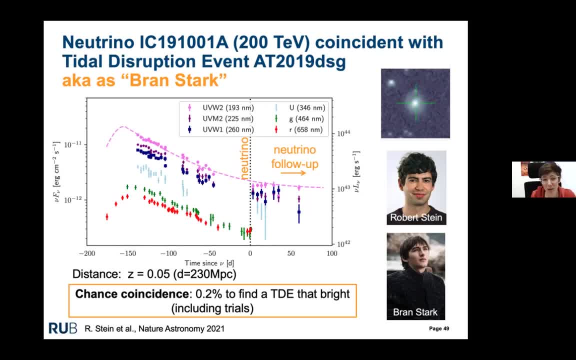 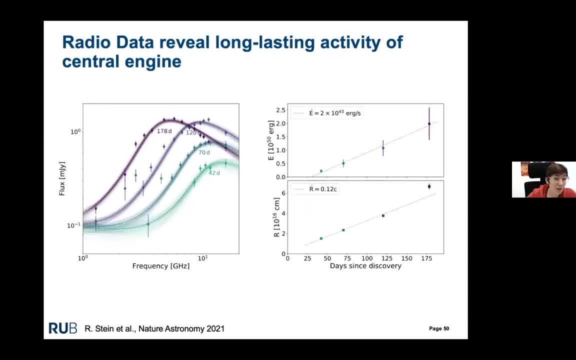 Naively, we would have expected that The neutrino would be somewhere close to the peak. So we took a closer look at the source And we looked at the radio data that was collected for the source, And the radio data actually reveals that there is some activity going on in the source. that 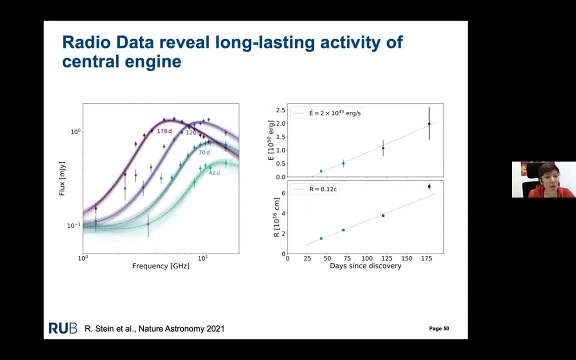 is lasting actually pretty long, until the time when the neutrino arrives, And you can see this in this part. This is not a light curve. This shows the frequency here And the time evolution is now color coded here. So you see over time that the neutrino arrives. 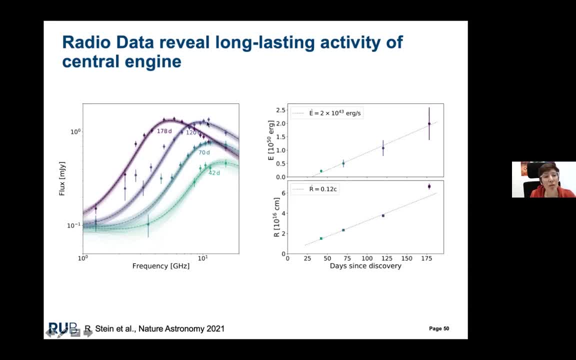 And you can see that actually the flux is increasing. Then eventually it's moving to low energies And from this we calculated the radius of the emission region and also the energy And you see that continuously over time there is still energy injected, which then convinced us. 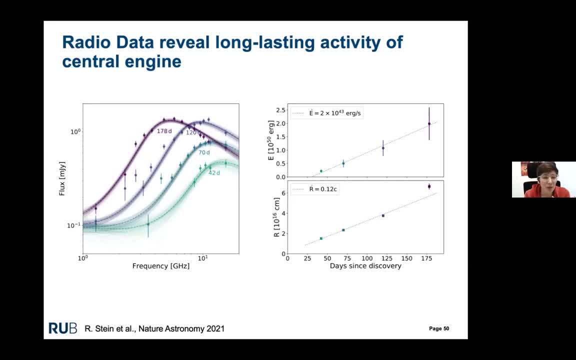 that it was actually reasonable to see the neutrino at later times because the activity was constant over time The neutrino could arrive. It could arrive whenever during that time. So yeah, we're quite excited about this measurement because actually it shows that there 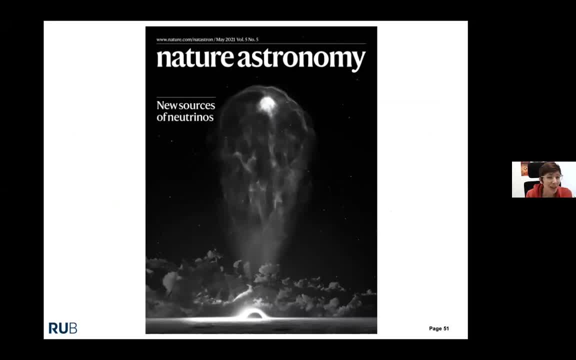 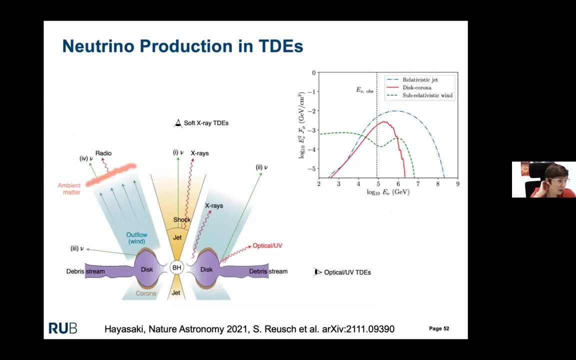 is a whole new source class out there, And it even made it to the cover of Nature Astronomy, maybe also because we have actually the nicest illustrations here. So where do the neutrinos actually come from? Following our more observational approach, we found out that 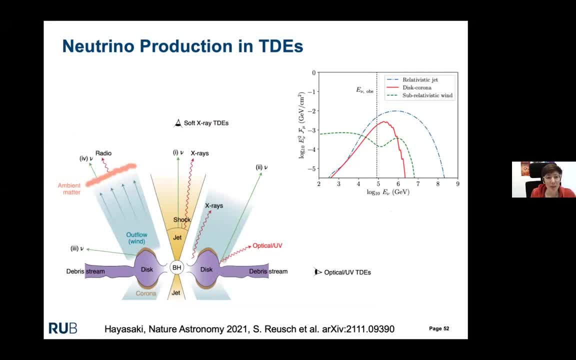 in the paper. there were several theory papers predicting neutrino emission from specifically that source or the sample of TDEs, And there's three major different models. So the neutrinos could either come from the disk itself, the equation disk, Or they could come from some hot corona around the disk. 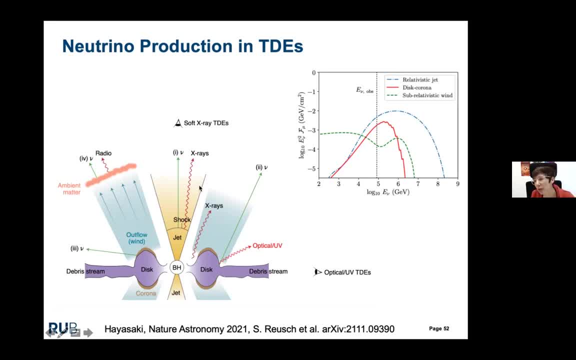 There could be a subrelativistic outflow Or there could be a relativistic jet, And in all of those environments the theorists argue that you would have high magnetic fields to accelerate the protons to high energies, And then you have photon fields as a target. 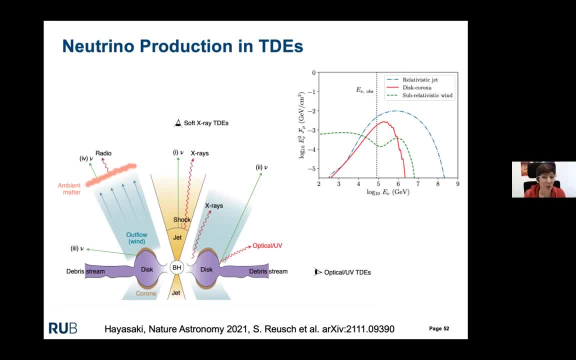 So the protons would interact and produce the high energy neutrinos And the different models would predict different neutrino spectra And you see this illustrated here. So the red one would be the disk corona model, The green one is a subrelativistic wind. 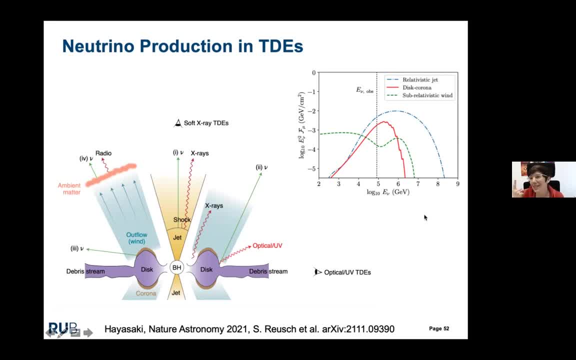 while the blue one is a relativistic jet. Of course now with a single neutrino, we are not able to distinguish those models, But maybe in the future, if we would see several neutrinos from the source, we could actually then compare it. 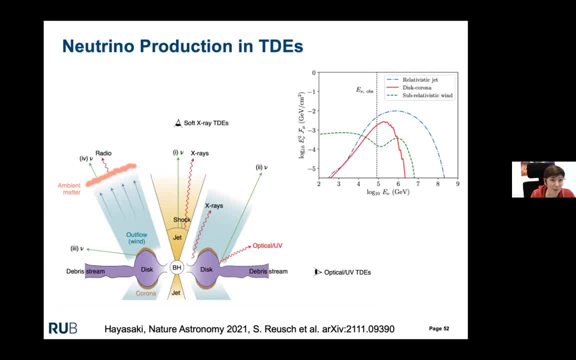 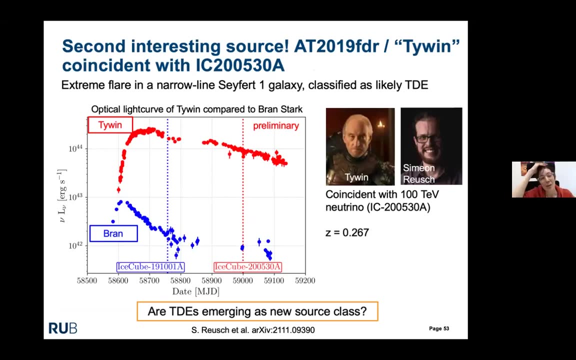 to the predicted spectrum. Even more exciting, this is not the only source we have identified. A little bit later, we found a second A candidate, And this is another likely tidal disruption event, coincident with the high energy neutrino that we also identified with our ZTF follow-up. 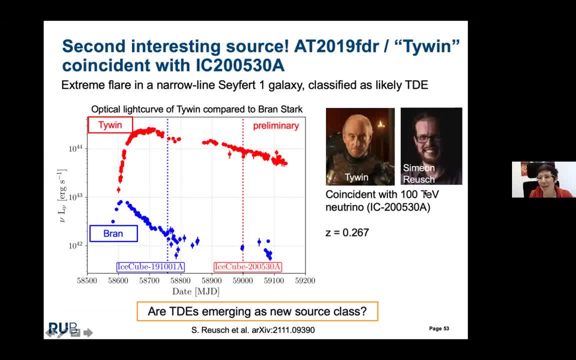 And this work was led by my student, Simeon, And maybe there is some similarity between Simeon and Tywin, which is the Game of Thrones nickname for this source. If you imagine that Simeon ages for 50 years. 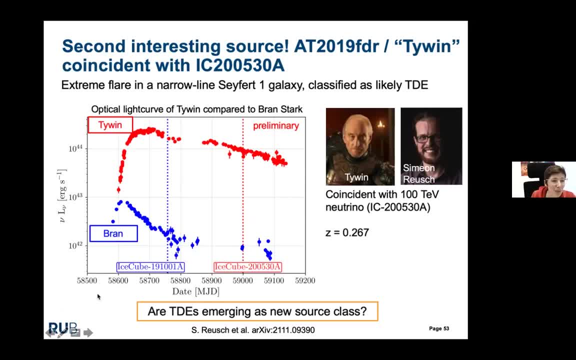 then maybe it would look like this. So this is a comparison of two neutrinos, Bren and Tywin. Yeah, I showed you, Bren. first You had the Lycophere And the neutrino arrived 150 days later. Now Tywin is much more luminous. 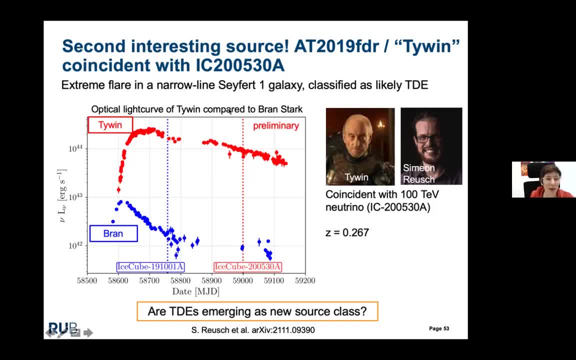 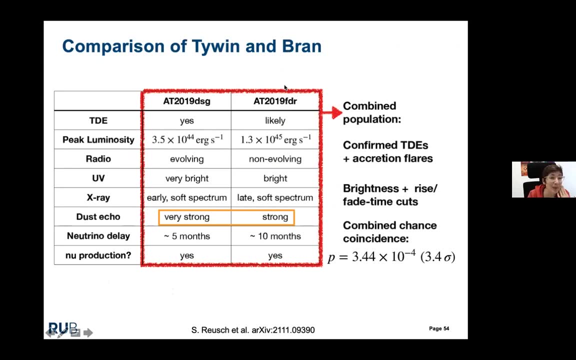 And the neutrino arrived roughly 300 days after the optical peak, So this is now an indication that maybe TDE's are emerging as a new source class. Yeah, We took a more Detailed look at those two different sources and compared them. 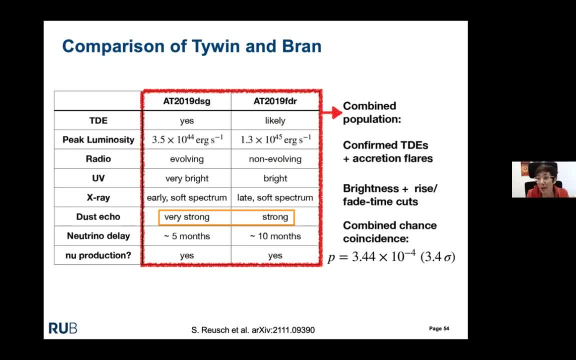 And we also calculated the now combined chance probability And we find that actually now finding two sources brings us to now above 3 sigma. 3.4 sigma would be the p-value in this case. But what we found interesting was that both of those sources have a strong dust echo. 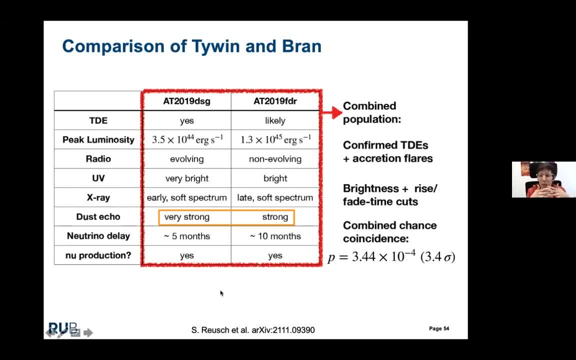 So what is a dust echo? So imagine you have the emission From the equation disk in optical UV And if there is a lot of dust around the source, then eventually this emission will hit the dust. So it would be a bit delayed because it needs some time. 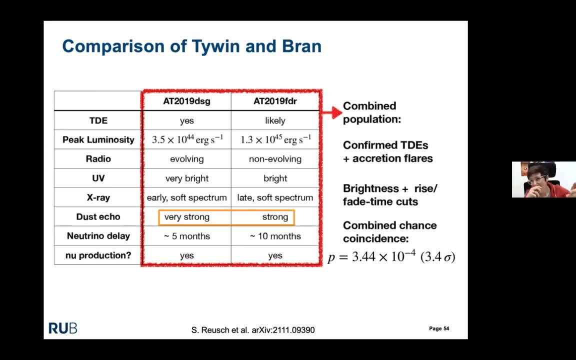 to go to the dust, heat up the dust and then the dust would re-emit the emission in the infrared. So that is the dust echo. So it's a peak in the infrared that is delayed compared to what we see in the optical. 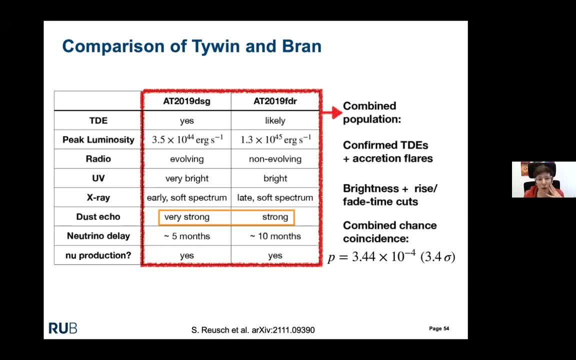 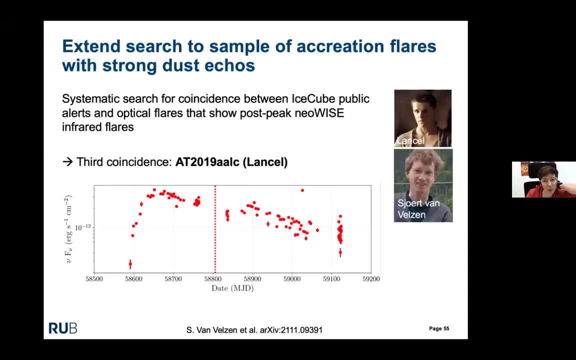 So we thought it was interesting that both of those sources show a really, really strong dust echo in the infrared data measured by NEOWISE. So our collaborator Schott van Lelsen did a dedicated search for neutrinos coincident with such flares that also show strong dust echoes. 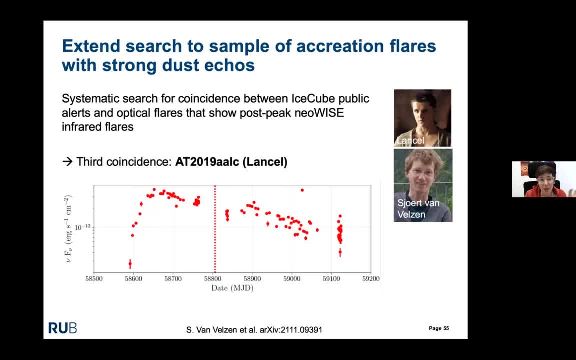 So he created a sample of optical flares that also show a post-peak infrared flare And in NEOWISE data, and correlated those flares with the public neutrino alerts, And he of course, found the two candidates that we had already identified. 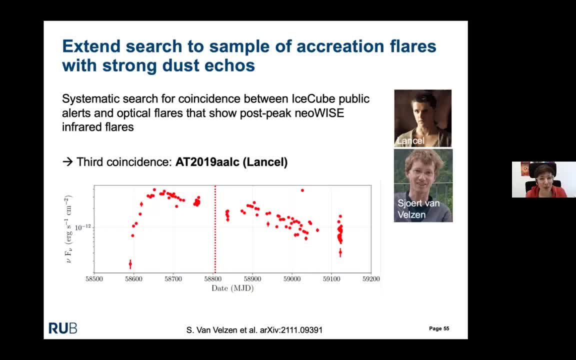 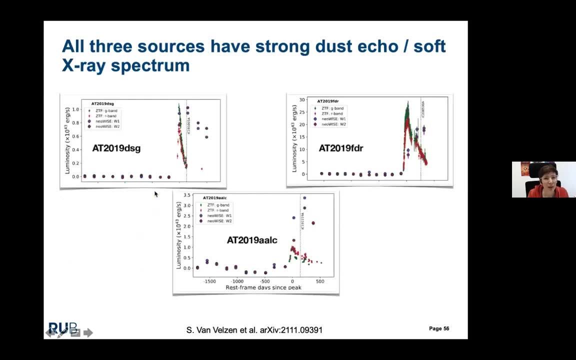 And he identified the third source that is called Lenzel in our Game of Thrones naming scheme. And here you see the optical light curve. So also here there was some delay of the neutrino compared to the peak. So this is a summary. 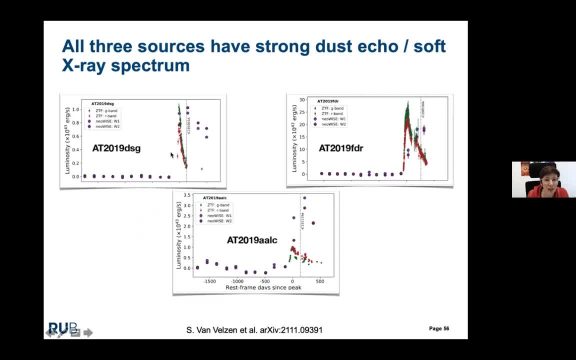 Showing all the three sources. You have the optical data from ZTF in the two bands, in red and in green, And you see the dust echo overlaid, So the NEOWISE data overlaid. So you nicely see that there's this huge jump, that 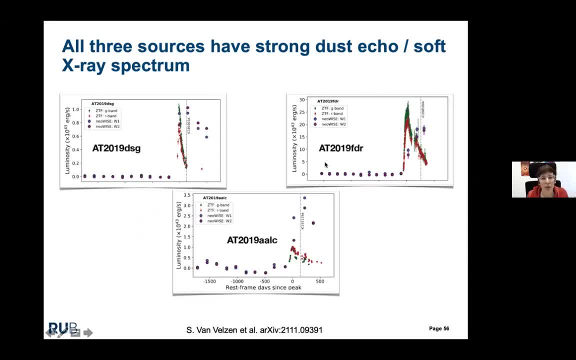 is usually a bit delayed relative to the optical peak. So this is for Bren, This is Tywin And this would be the new source, Lenzel, that also has the optical peak here, And then the delayed peak in the infrared And now, combining all the three sources, 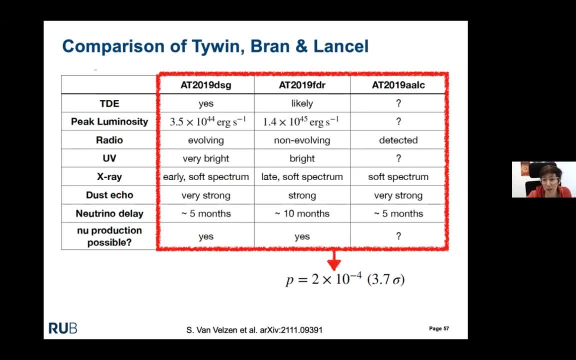 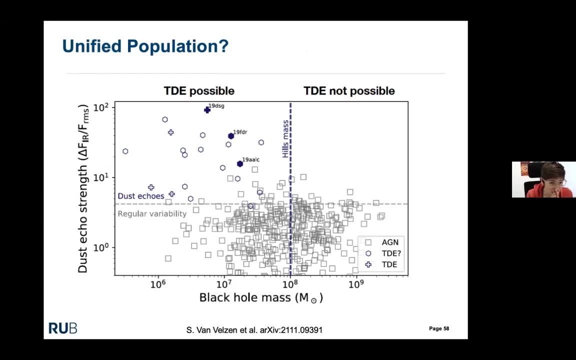 Also, Schott calculated the significance And he now finds an even increased significance of 3.7 sigma. So maybe this is some unified population of sources. Yeah, Just so we can see what we found. So what we want to do is not to just find a few. 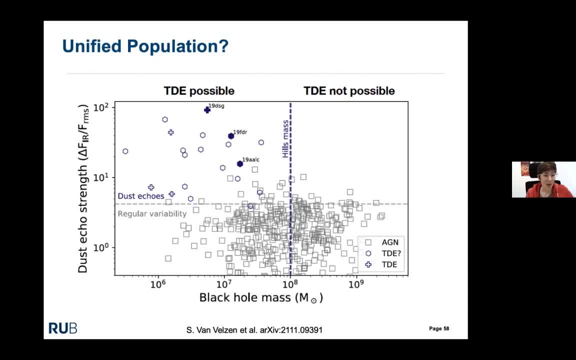 but some kind of unbalanced distribution of the particles that are able to accelerate protons to higher energy descent and then those protons interact and produce neutrinos. And now look at the distribution of the black hole mass of the objects producing this accretion flare. 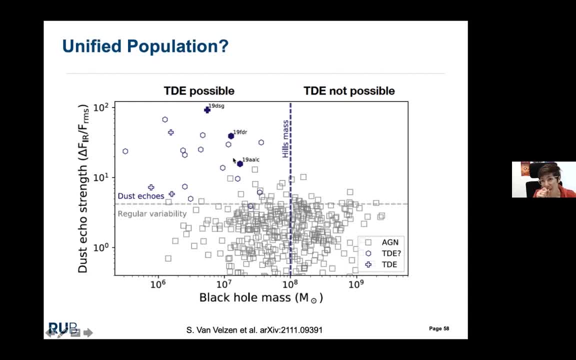 And here he plots the dust echoes, strength AGN detected by ZTM that also show such a dust echo. And you see that all the TDE candidates are actually in this upper part in the plot. And those third sources are the three sources. 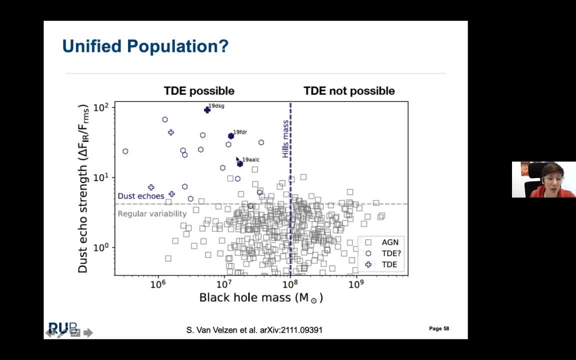 we found incident with high energy neutrinos. So he defines a cut here where below this cut, because of regular variability and the strong dust echo, he would define everything that's above a certain threshold. The other line you see here is the so-called Hiltzma. 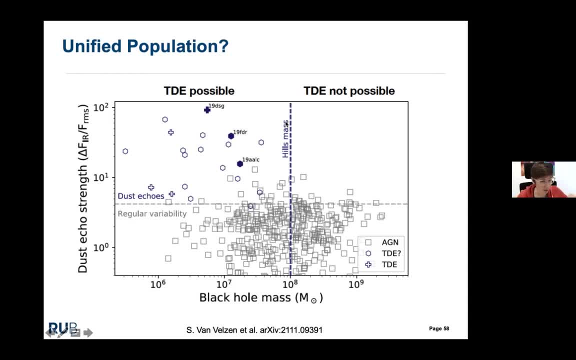 So eventually, if the black hole gets too massive, you wouldn't see a tidal disruption event anymore, because the event horizon eventually becomes bigger than the tidal disruption radius. So the star would actually just disappear and you wouldn't see the disruption. Yeah, so interestingly all our candidates lie up here. 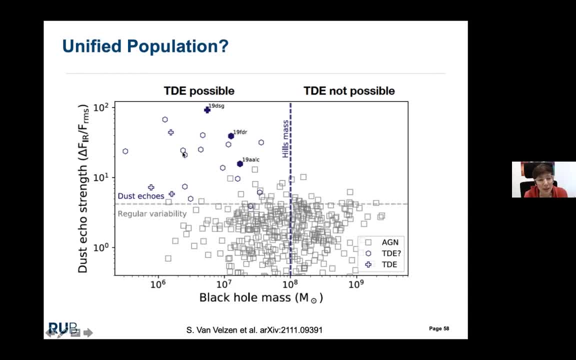 So maybe that is really a unified population. And now the next step is to really do a targeted search for neutrinos, using not only those events but really the full sample of neutrinos detected by IceCube to do a dedicated search, a stacking analysis. 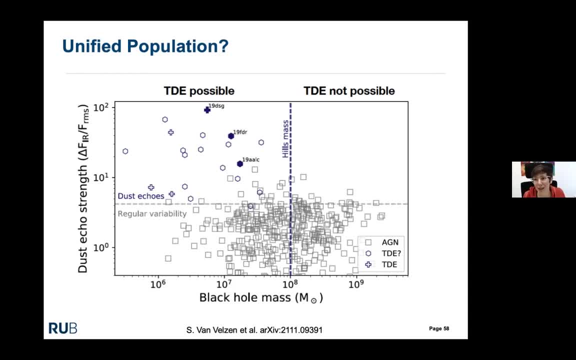 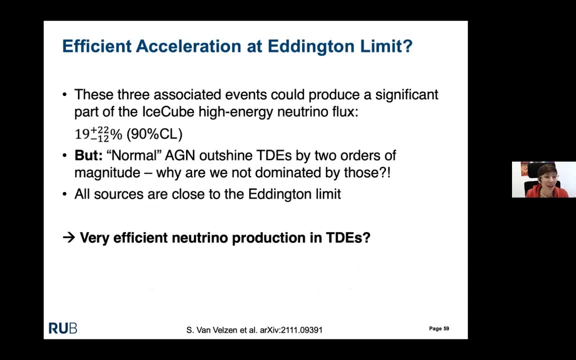 combining all those sources and see if we actually find an even stronger signal from those sources, basically testing this hypothesis that this is an interesting population of sources capable of producing high-energy neutrinos. Yeah, so we find those three interesting events associated with high-energy neutrinos and we calculated 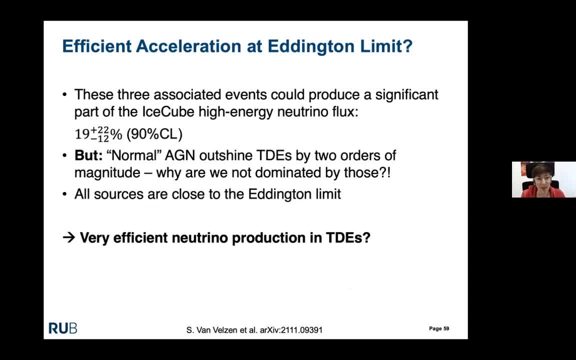 that they can actually produce a significant part of the IceCube neutrino flux. Not all of it, but yeah something at the 20% level. But keep in mind those are like large, large uncertainties, because we're talking about a small number of statistics here. 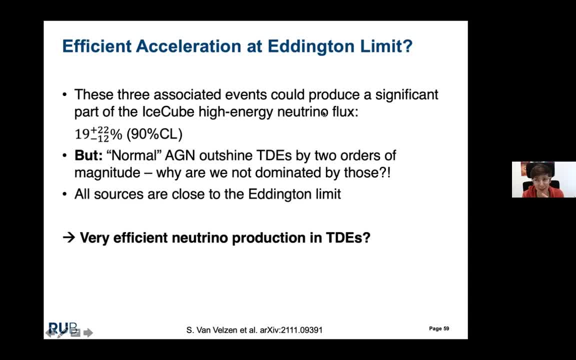 However, what is really puzzling about this finding? if we believe that this association is true, then it is not really clear why we see neutrinos from tidal disruption events but not from AGM. But because the total energy output by AGM 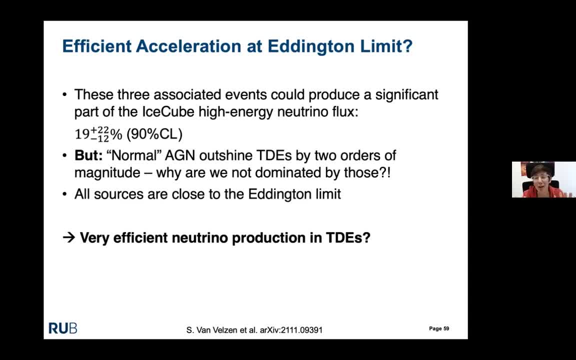 is two orders of magnitude above the energy output of tidal disruption events. So we can't really tell: Yeah, So we should really be dominated by AGMs and not by tidal disruption events, but we somehow see the opposite. So what Schott proposes as a solution for this problem? 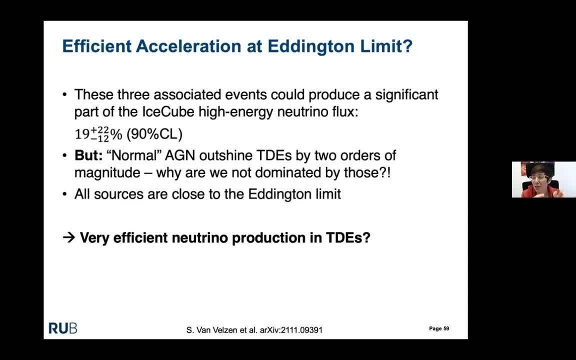 is that there has to be some very efficient neutrino production going on into these that you would not have in an average AGM And maybe this is connected to the emission being close to the adding limit or above adding limit For those accretion flares and tidal disruption events. 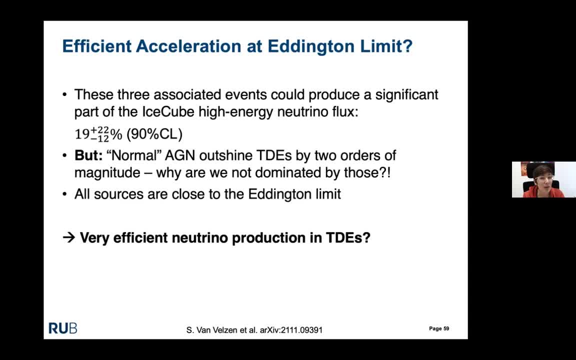 for the three candidates that we have found. So maybe there is some efficient acceleration going on at the adding limit. that could explain why we see neutrinos from tidal disruption events but not from regular AGM. So this is really something we could throw already now. 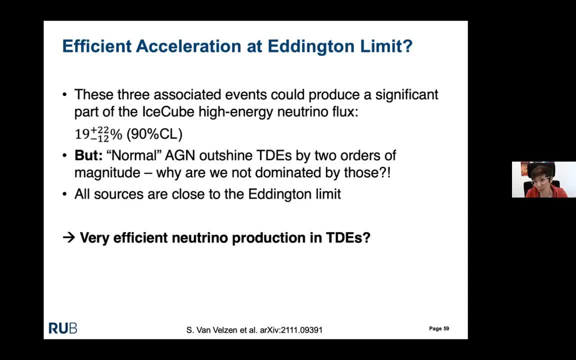 with existing ice cube data, We can use the sample and look what's happening. It's not a very good idea to use the sample for the next generation of the two telescopes And it's a very good idea to use the sample for the next generation of the two telescopes. 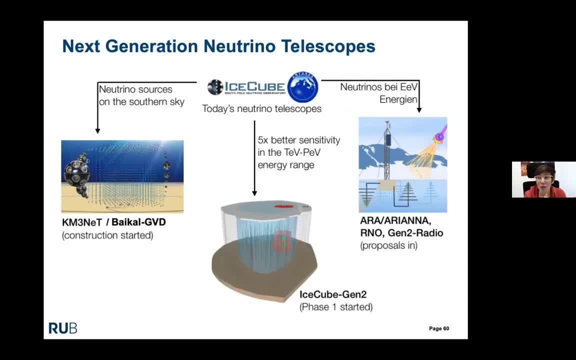 So we have two instruments currently under construction in water: There's the KM3 net detector under construction in the Mediterranean And there's the Baikal GVD detector under construction in Lake Baikal in Siberia. In addition to that, there are also. 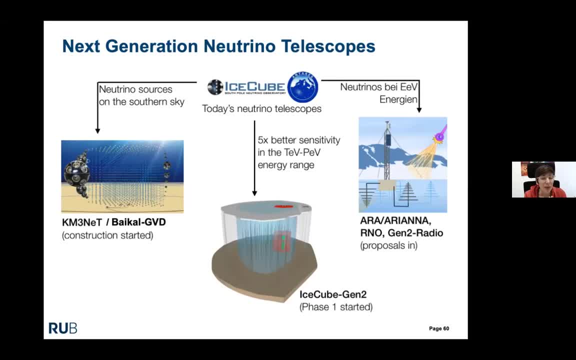 plans to extend the detector at the South Pole And that would be called IceCubeGen2.. That would be in ice detector almost 10 times bigger than what we have right now with IceCube paired with the radio surface detector on top of the surface of the ice. that 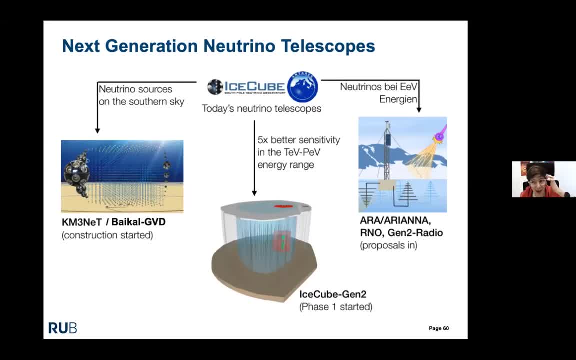 would extend the sensitivity also to higher energy. So really, in the future We will be able to detect much more neutrinos And of course, there will also be new follow up instruments, such as LSST, that will allow us to perform a similar search. 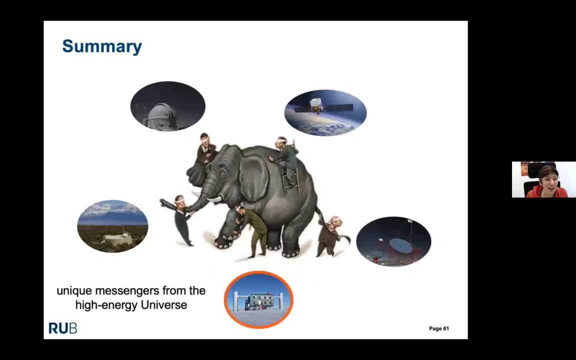 but be much more sensitive. So, in summary, I hope I could convince you that neutrinos are really unique, interesting messengers from the high-end universe. There is this tight connection to cosmic rays where neutrinos could help us to identify the sources. 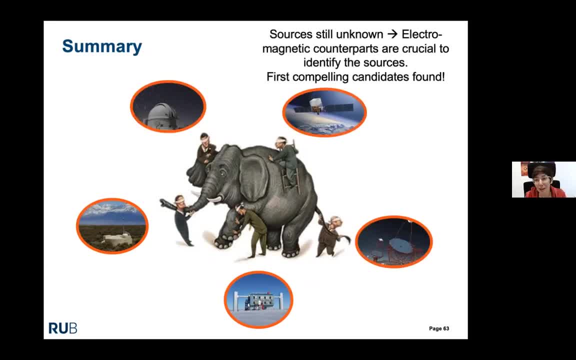 And I think I showed that most of the sources of the diffused neutrino flux are currently still unknown. But searching for the electromagnetic counterparts is really the key to identify the sources, And I showed you that we have some first compelling candidates identified. There is the Texas blazar, where we found a high-energy neutrino. 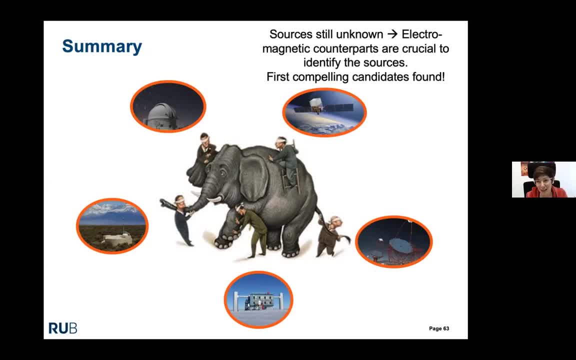 from that direction And several TDE candidates that are promising sources for production of high-energy neutrinos. So in the future I guess the task of the experimentalists is to probe also other source classes and go even deeper on the ones that we have identified. 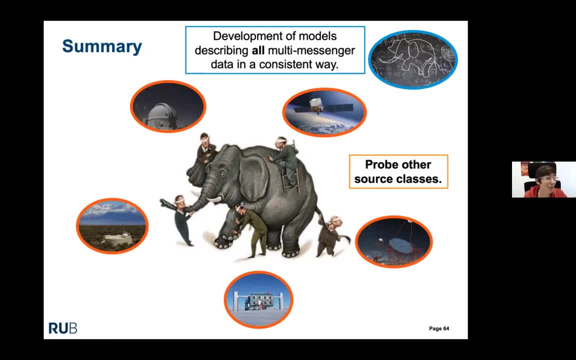 as potential candidates now, And theorists have to develop consistent models that can really describe all the multiplicities. So with that, I think I'm going to end my presentation, But I'm going to say goodbye now, Thank you. Thank you for watching. 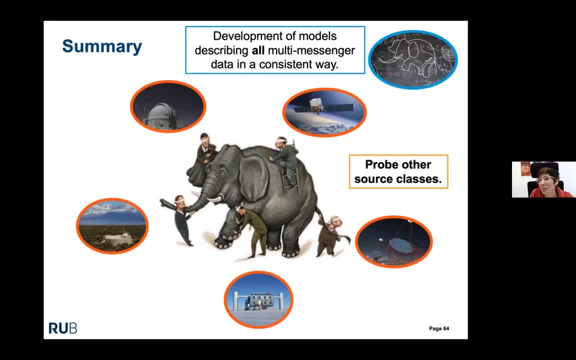 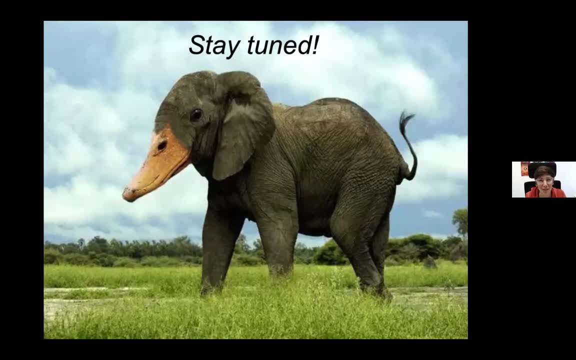 And I hope you enjoyed it. I hope you enjoyed the video And if you liked it, please don't forget to like and comment and subscribe and share, And if you didn't, you can follow the link in the description below And thank you for watching. 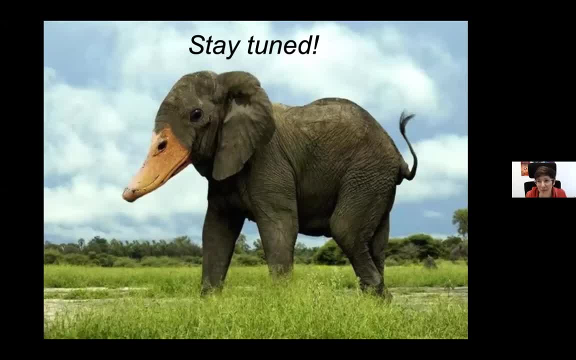 I hope you enjoyed it. I hope you enjoyed it And thank you for watching. And thank you for watching. Thank you for watching. I hope you enjoyed it. Bye, Bye. Thank you very much, Anna Irina. am I supposed to share this part? 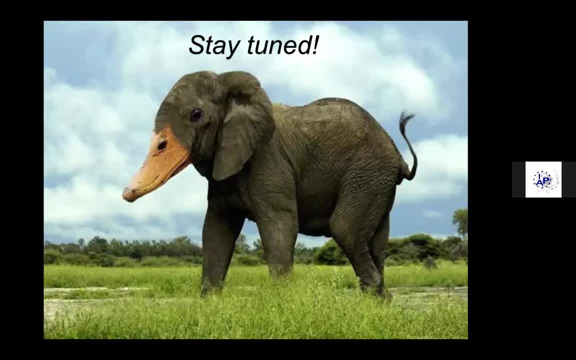 Yes, if you. Okay, great. Okay, thanks a lot, Anna, for this great talk. Do you have any questions? You can either raise your hand or just speak up. Okay, actually I had a question in the meantime. So thanks very much for this inspiring talk. I had a question about this delay time between the optical peak and the neutrino signal. 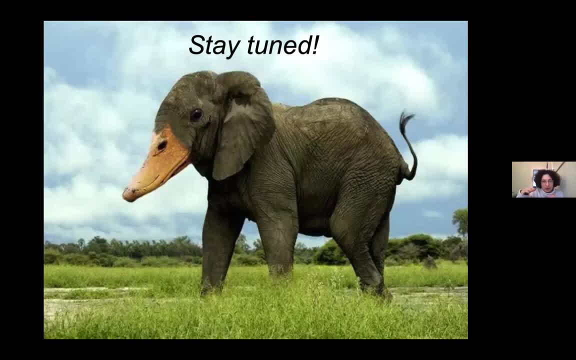 Is it just because the neutrino signal it's kind of uncorrelated with the optical, So it's, Is it just a rush at any time, or is there a physical significance of this 150 days or 300 days delay? Yeah, so, naively, I think naively, we thought that the neutrino mission should be correlated with the optical. 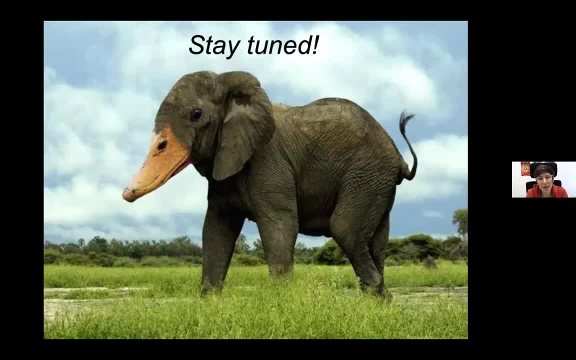 But now, yeah, the radio gives us some indication that there is actually still activity in the central region, even at later times when the optical already starts to decay. Okay, And there was also some model trying to explain that with the activity of the jet and that eventually something 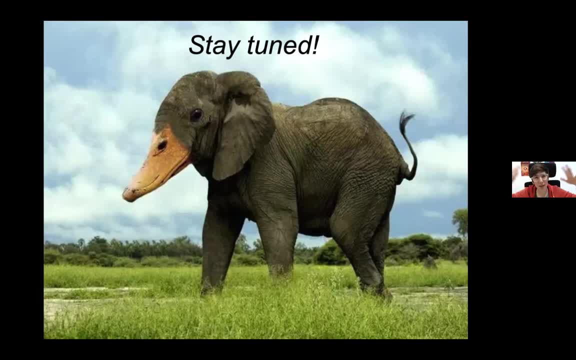 So the target photons would increase, and Yeah, but that's. They could somehow fine-tune a little bit when you would see the peak in the neutrino production. I'm not sure if I have this in the back up. Let me check. 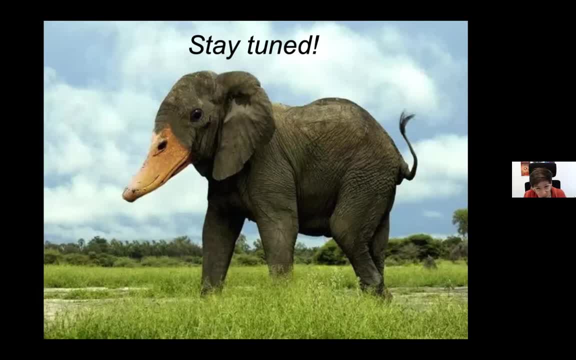 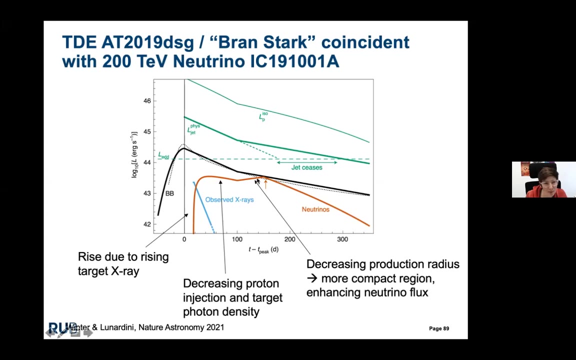 No, unfortunately I don't have it. I don't have it here. Yeah, As I said naively, it's not what, Oh, no, Here it is, Let's see. Okay, So yeah, in this model they can actually manage to get this kind of small bump in the neutrino light curve at the time where we see the neutrino. 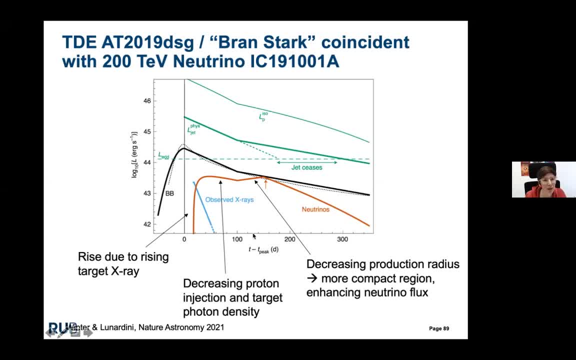 But I think this is a bit fine-tuned here. So you have a rise in the X-ray target And at the same time the proton injection is decreasing, And somehow, when you combine that, you can make it work. Wouldn't we expect another peak in neutrinos just right after? I mean around, I think it's 10 days or something. 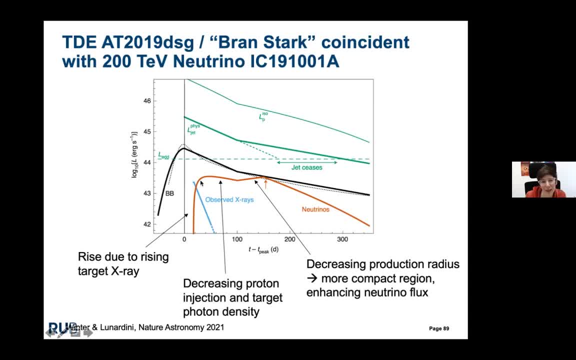 Yeah, they have two peaks. Yes, But I guess, like in this region, it looks like it's more or less constant, right? So then you could have the neutrino any time there, right? You have to keep in mind that we saw one single neutrino here, right? 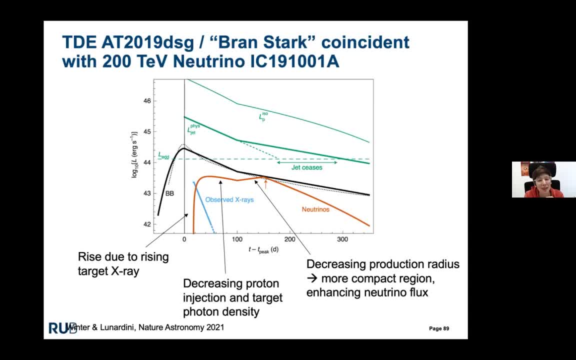 So probably when you calculated the expectation value from a single source like this, it would actually be below one. But there is something called the Eddington bias. So now imagine we. We monitor the whole sky in neutrinos all the time, right? 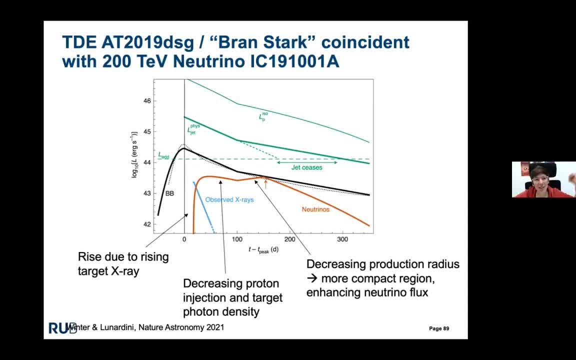 But there is probably, let's say there's- a thousand tidal disruption events And each of them has an expectation value of 0.01.. And then eventually one of them will do a Poisson over fluctuation and send out one neutrino. 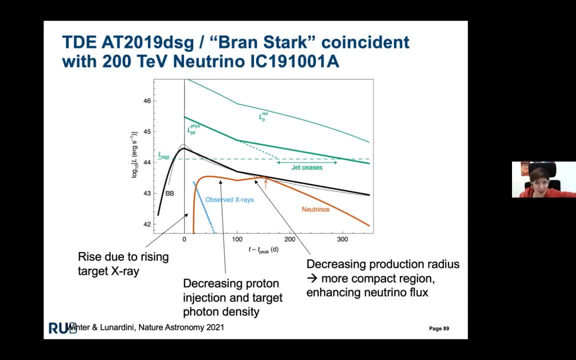 And this will be the one that we observe and point our telescope at. So, okay, okay, So you have. Yeah, we see only one neutrino, so we can't really get a neutrino light curve And probe a model like this. 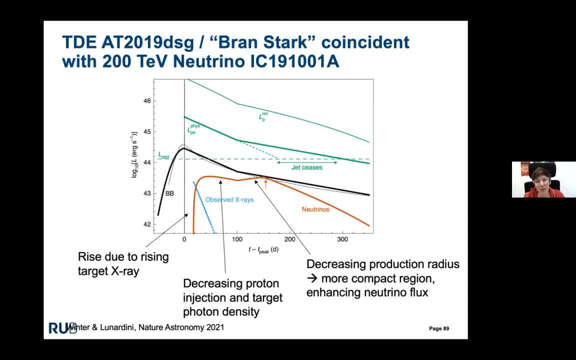 That's the problem. Building on this, I guess you performed archival searches in these directions, in neutrinos, did you? So we're planning to do a new archival search. There was one done more than two years ago, So this was before ZTF. 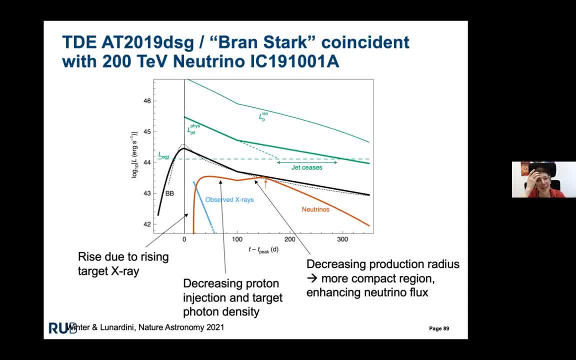 ZTF actually started to produce a nice catalog of TDEs. That was also done by Robert. So he used all the TDEs he found in the literature and looked for neutrinos in the archival data in the stacking analysis. That also included the three jetted TDEs. 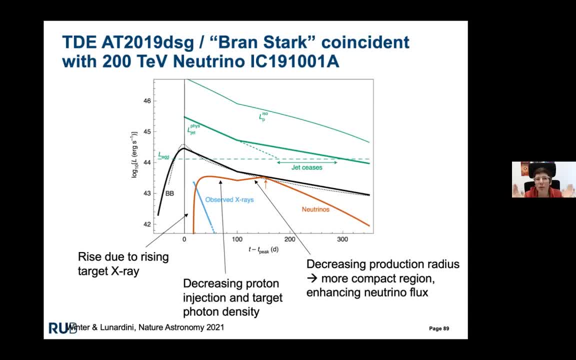 However, at that point we used a generic time window. We didn't really know what we were looking for, So we used a 100-day time window. So really, if there is also delayed emissions, we maybe would have missed it. 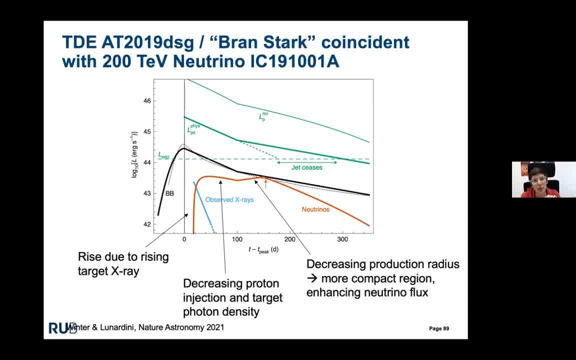 And also it was a small sample of TDEs that we looked at Because it was before the time of ZTF. We have another analysis in the pipeline But, as you know, in the big collaborations it just takes a while before you're even allowed to look at the data. 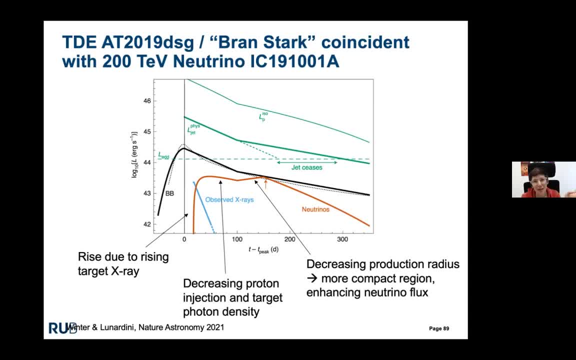 So we do blind analysis. You have to do a study on Monte Carlo data presented, It will be reviewed And then eventually you're allowed to open the box. So we're planning two different searches, Actually one just using all the optically detected TDEs from ZTF. 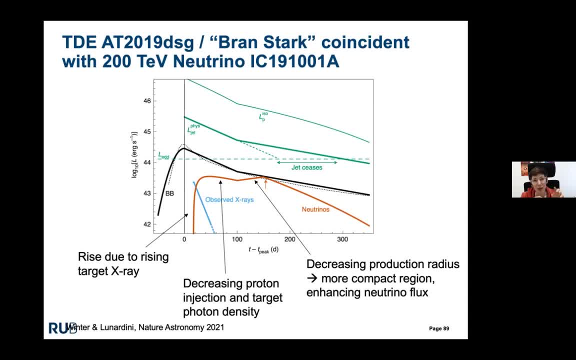 And then we want to do another one using those accretion flare sample that Short used in his search where he discovered the third source. So those two different ones we plan to do. OK, Any other questions? I think it was crystal clear. 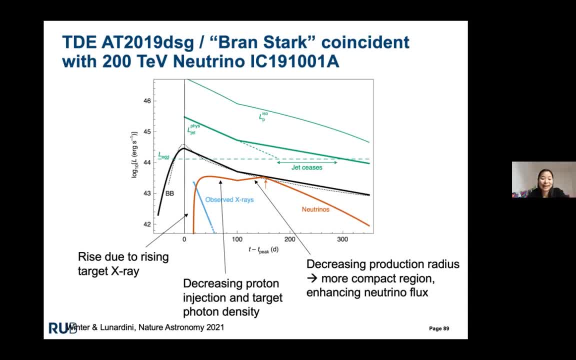 I hope it was. Don't be shy to ask questions. I'm happy to try to answer them. Actually, I found this very pedagogical and very clear. Can I ask one more each? So when you talked about The coincidence between 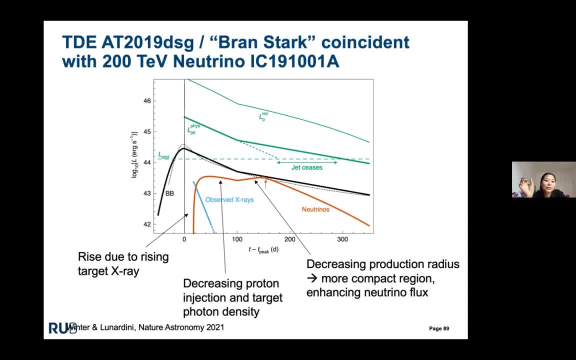 You put a number on the coincidence probability of two TDEs being detected. What's folded in this number? How would you actually calculate this? Yeah, So we had to define a sample. So we, Yeah, We looked at So what goes in there? 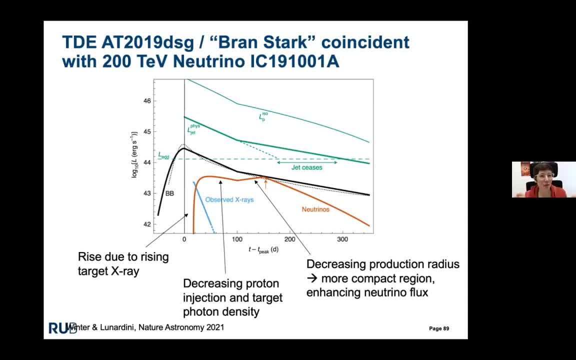 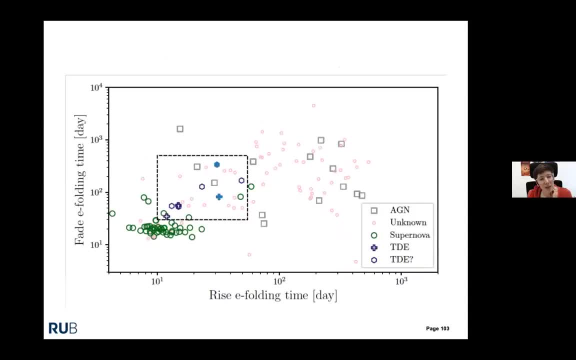 It's like: how many follow ups have we performed And how many square degrees did we cover in the follow up? Yeah, That goes in there, And then we defined a sample using this. So this is sources detected by ZTF. And yeah, we require to find a flare that has a certain shape. basically, 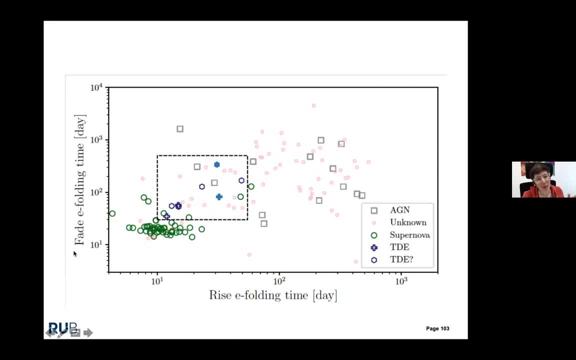 So we would not take into account, Take into account something that is like a super long flare or a super short flare, So we can By this, Yeah, So basically everything in this box we would have called like an interesting event, And then we can calculate how many would we have expected in the area that we cover in. 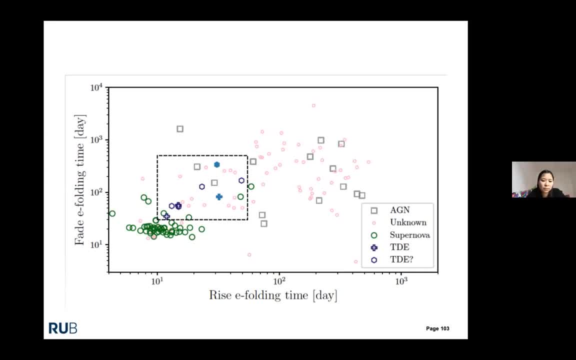 the follow up. Okay So, And what's the? What's the size of the? So, Oh, no, Okay, Sorry, Sorry, Sorry, Okay. So here is, This is just the How we, How we would select the. 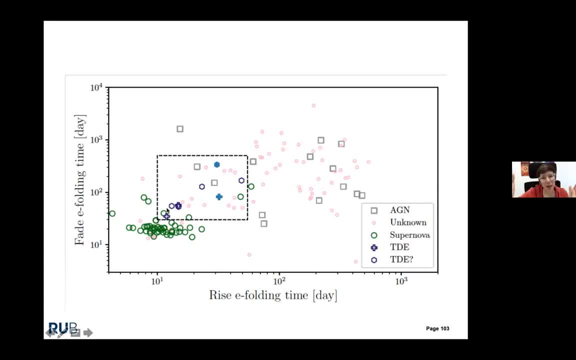 So, based on the light curve, basically we define a sample of flares that we would consider tidal disruption events. right, Because you can, If you use everything that is flaring, you would also include supernova and other ADN activity. 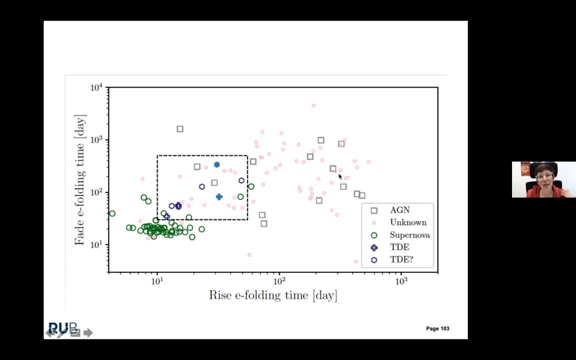 So we basically fit something to the flare and then we use the rise time and the decay time to define that window. And yeah, the other ingredient is: how many square degrees did we cover? So we had to include all the follow ups that we have performed. 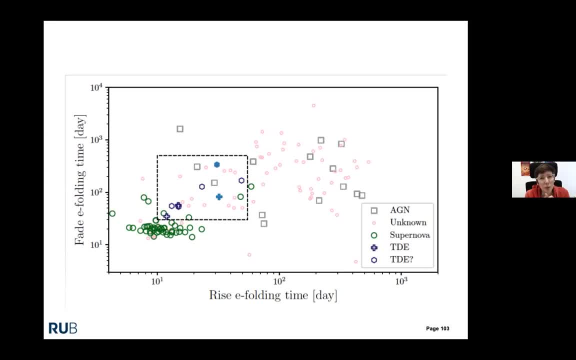 We do not follow up every alert from IceCube. We make a selection that either has high signalness- about 50%, and we would all the time follow it up- Or if it has low, Okay If it has lower signalness. 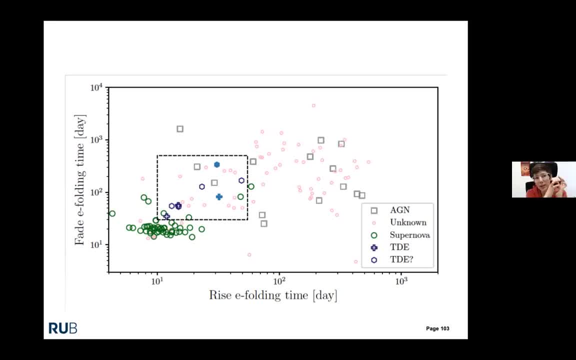 Okay, If it has lower signalness but a small localization, we would also follow it up, Because some of them they are like a 30% signalness but have a 50 square degree area in the sky, right, Those? we do not even bother to follow them because we would find so many things and 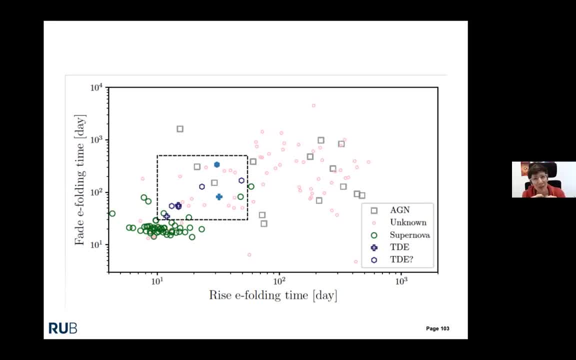 that would kind of ruin everything we would find because we have this large area. So I don't know the number. from the top of my head I think it's something like 150 square degrees. that in total we covered All the follow ups that we have done. 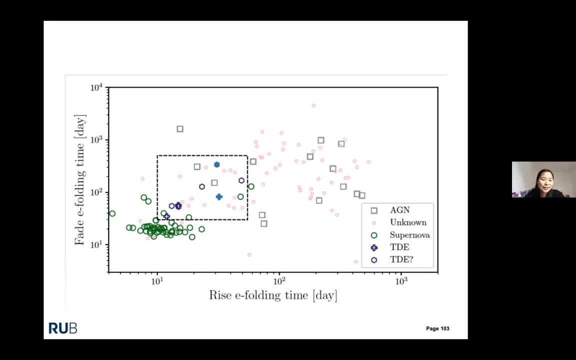 Okay, Okay, Thanks. Everybody's being shy. Okay, If I don't know, I will just ask one last question. So you just mentioned in the end that you would like to search for other sources, I guess among the possible candidates that you described previously. 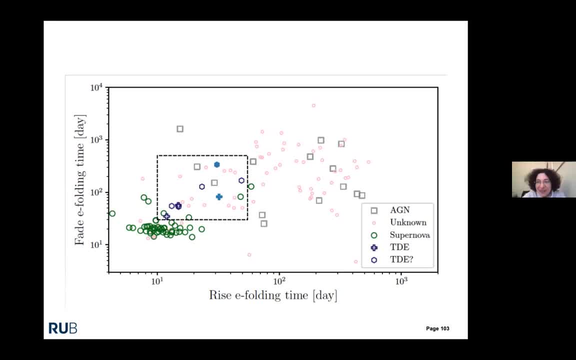 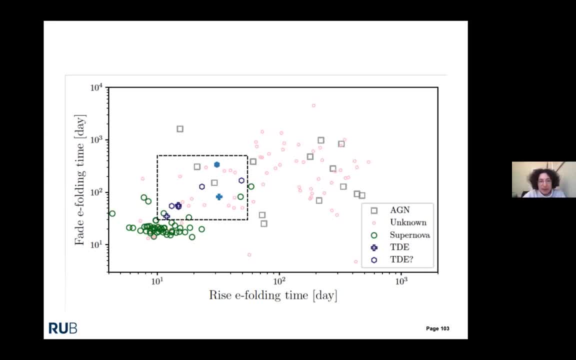 Yeah, Yeah, Yeah, Yeah. I do want to make one more question then. Can you maybe say a few words about which kind of like other specific programs that are put in place to search for, for example, this supernova that interacted with the?